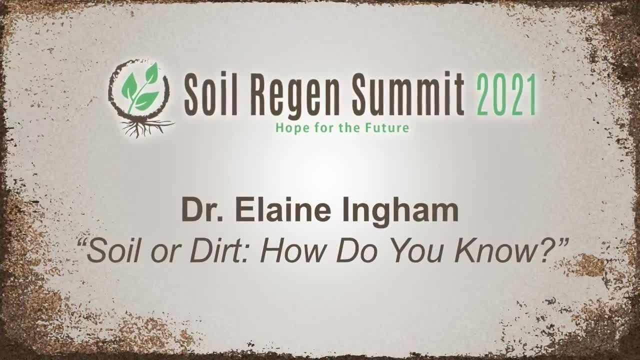 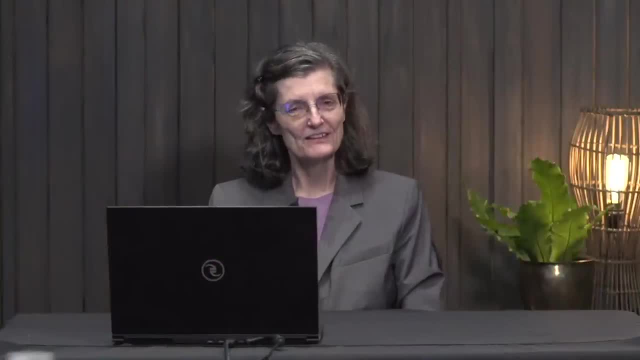 Good day everybody. Hope you've been having a good time at the Soil Summit listening to all these great talks by all the different speakers. So today I'm going to start out with a little bit more discussion about what is dirt and what is soil. So again, my favorite. 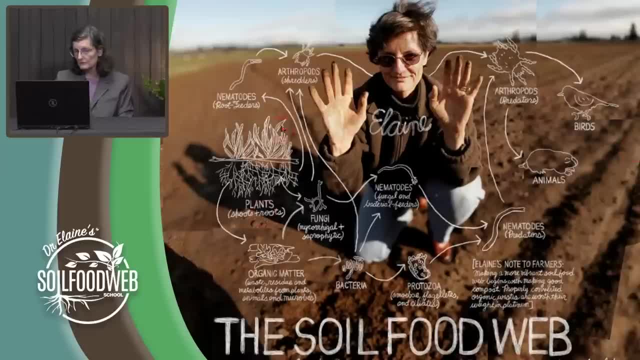 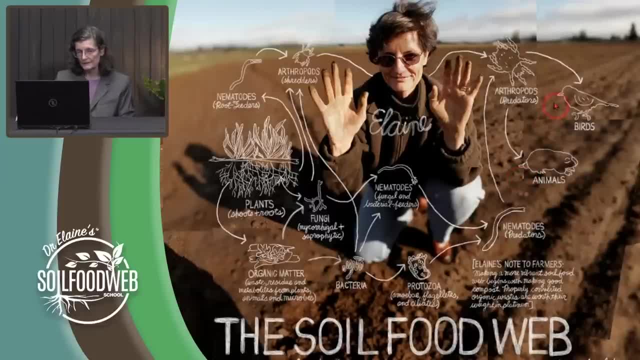 If it was soil, it wouldn't have a compaction layer. Your organisms will build that soil structure and it will not compact as long as you're treating it right Now. you go in with some fertilizer, you go in with some soil. you go in with some soil. you go in with some soil. you go in with some fertilizer. you go in with some soil. you go in with some soil. you go in with some soil. you go in with some fertilizer. you go in with some soil. you go in with some soil. you go in with some soil. 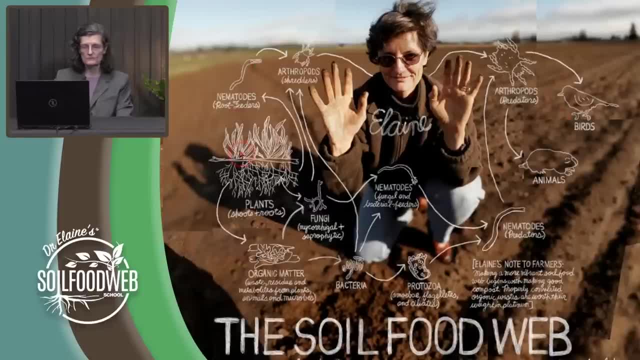 you go in with some fertilizer, you go in with some soil, you go in with some soil and you're going to be killing the biology in the soil, And now you're starting to turn it into dirt. How fast can soil be turned into dirt? Well, every time you plow, every time you till up this soil, you're slicing and 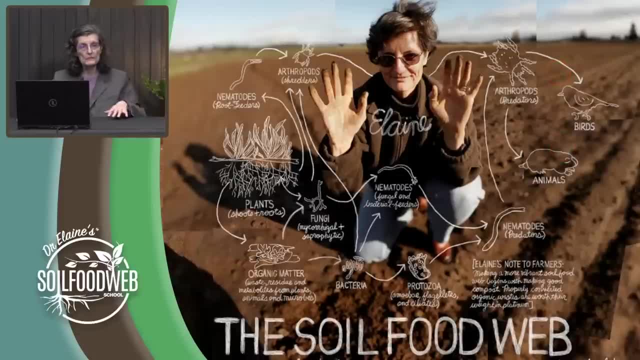 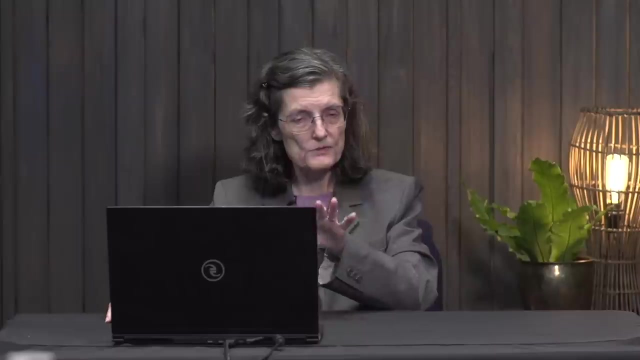 dicing and crushing the organisms that you need to maintain structure within the soil, So you can't be tilling. We want you to become no-till or minimal till. You know, certainly if you have rows out here, you can put a furrow down the row for just a small space on the top of that bed. 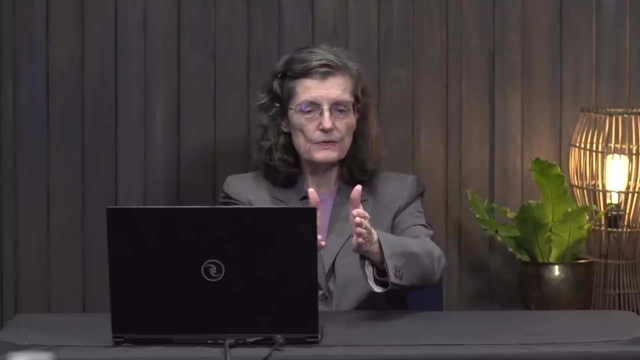 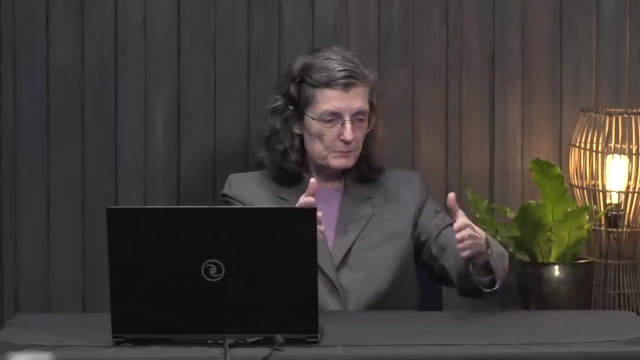 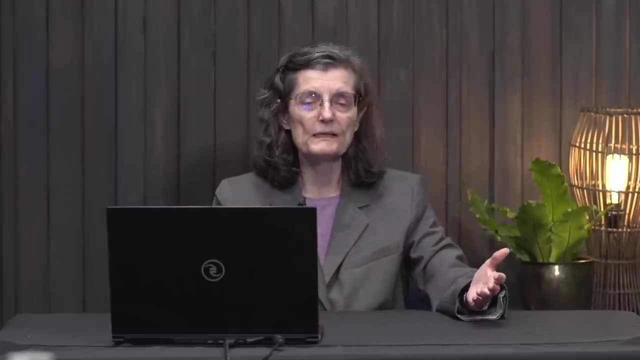 or in the soil. you just have the furrow and then you have a driving row or a walking row right next to that and then you would have another furrow. So there's plenty of space for you to be putting in perennial understory ground cover kinds of plants. We don't want those plants to be growing more than. just maybe a couple inches, depending on what crop you're growing. You might want it pretty much flat to the ground, or, if you've got a crop plant that's pretty tall, you could let it be six inches, Depends on the precise crop that you're trying to grow. We want you to put in perennial low-growing plant. 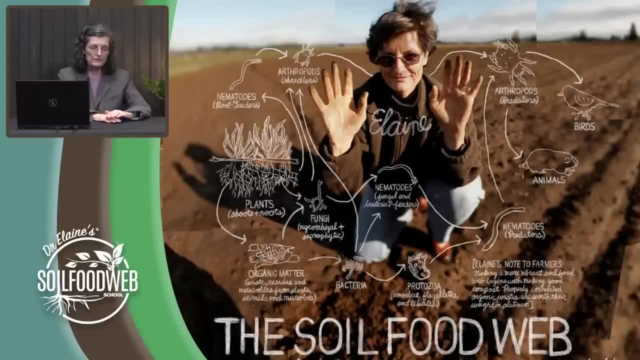 species cover, plants or ground cover, whatever you want to call them- that are perennial and they will always be putting exudates out into the soil to keep your good organisms alive. through the winter perhaps, especially if you don't have a very difficult crop, The soil doesn't freeze at all, or freezes only once or twice. Those plants may well survive. even a freeze or two before they succumb to the winter. Then they'll have to regrow from a crown come the next growing season. You don't have to keep buying seed if you're putting in a perennial plant. So you buy the mixture once. maybe you see that one or two of those species of plants didn't. get through a winter. so you over seed with something else. It's not very long until you have the system, the soil, completely covered, You know. so you put your start in. you're going to do do the furrow, drop your seed or drop your seedlings in. they start to grow, and pretty soon. they're up over your cover plants, shading those cover plants. You didn't have to go and find an herbicide to knock those cover plants down. You don't have to. You mow them and cross your fingers that you're going to be able to crimp the nitrogen fixing. plant that you added in with your mixture. Hope and pray that the vetch isn't going to climb up on your cut on your crop plant and cause problems. So we need to start thinking about shifting away. and oh yeah, these are perennial plants. Emphasize that you don't have to keep buying seed for them. 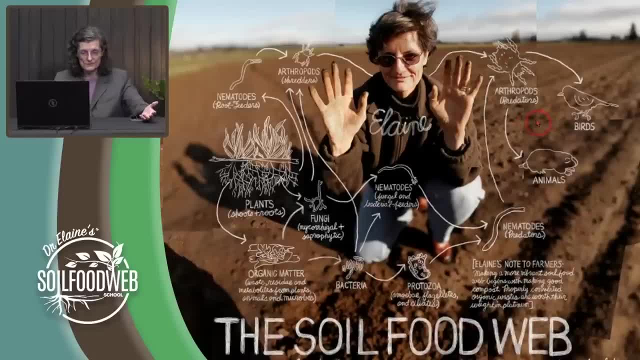 So let's start. Let's protect the soil surface from raindrops. One of the most compacting factor there is in agricultural production is rainfall from the sky, because where that drop of water hits the ground, it's causing compaction, typically somewhere around three inches deep into the soil. so 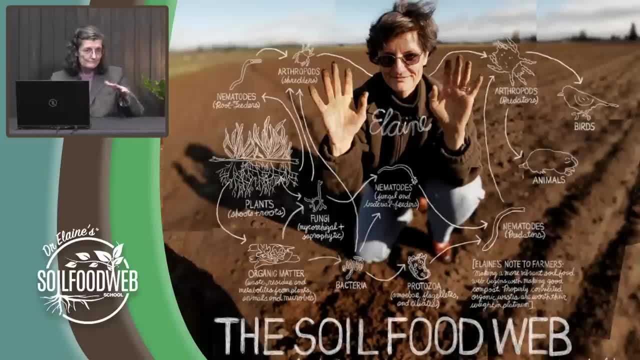 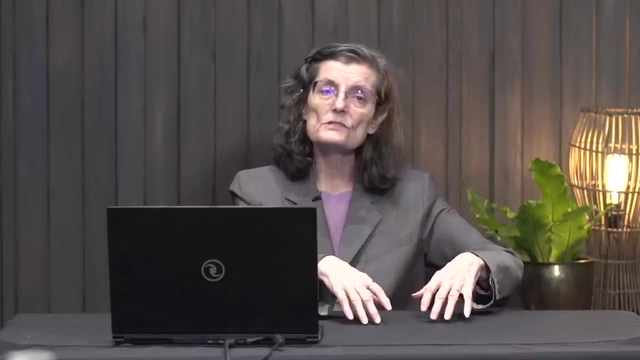 four to six inches. So you have to deal with the compaction that's been produced by the fact that you don't have your soil covered In the summertime, as water evaporates and it's pulled to the surface, bringing with it all of the soluble nutrients that might be in your soil, but when that water evaporates off into the atmosphere, those salts are left as a layer on the surface of your soil and it's going to cause harm to, though to, your plants. High salt levels are deadly Evidence. anybody who tries to drink salt water when they're out on the ocean will surely die. 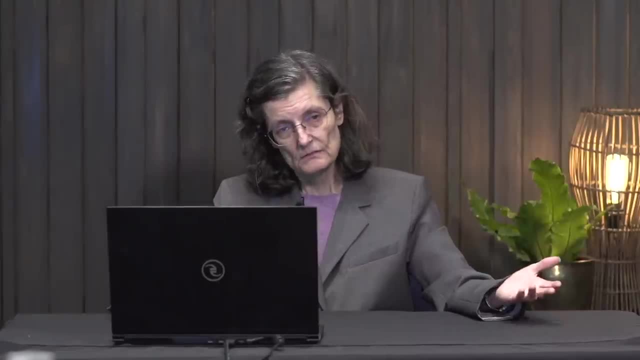 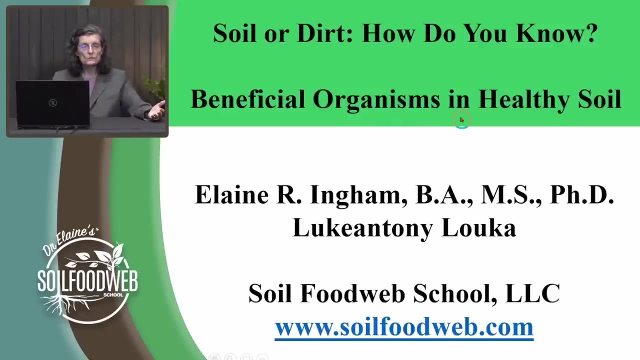 So we want to be aware of all of these factors. so you understand this soil, or is this dirt? Well, look at the beneficial organisms that occur in healthy soils, and so we talked about them. We talked more about the function yesterday than now. particular aspects of the beneficial organisms. 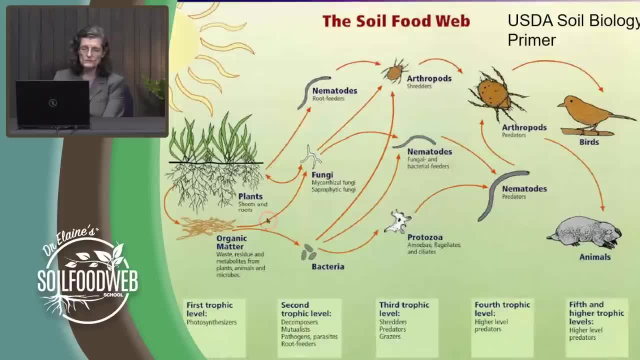 But again we're. we're talking about this food web. and where do you do these organisms fit? in dirt, What do you have present in soil? so hopefully, from yesterday you'll understand that these organisms are. of course you know you've got to have your plants. 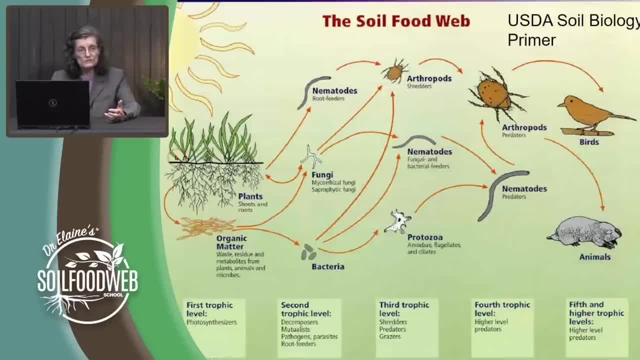 you have to have your dead organic material, so the residues that fall into the surface of the soil you will. you see that layer and you want that layer, the decomposed Quite rapidly so that the fungi are doing that. you know that the fungi are doing their job. 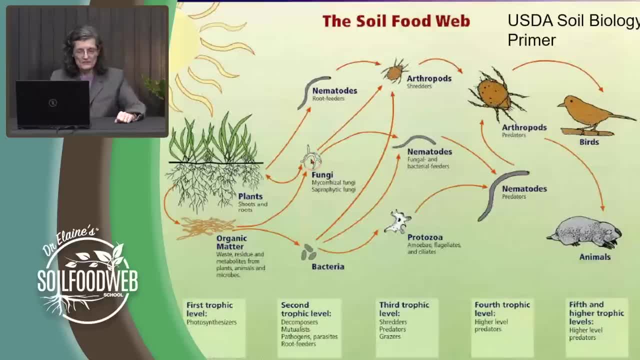 So one of the things I forgot to mention yesterday were the mycorrhizal fungi here, and we'll be looking at some of those today. How do you identify those? How do you make it easy for you to figure those particular colonization in the root systems? How can you measure that? So, 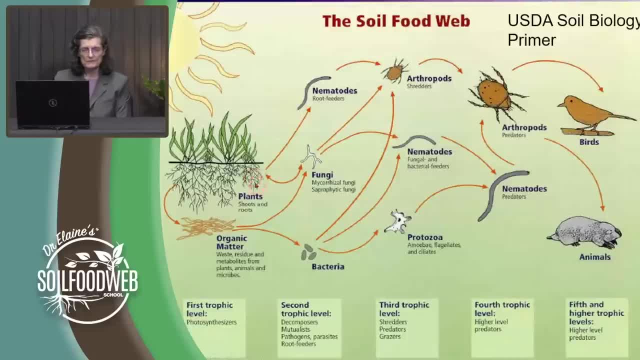 looking at that interaction between plants and mycorrhizal fungi. So fungi, the bacteria in the fungi, the protozoa, the nematodes, the microarthropods, the higher level predators, which someday we will get around to expanding those groups and learning even more. 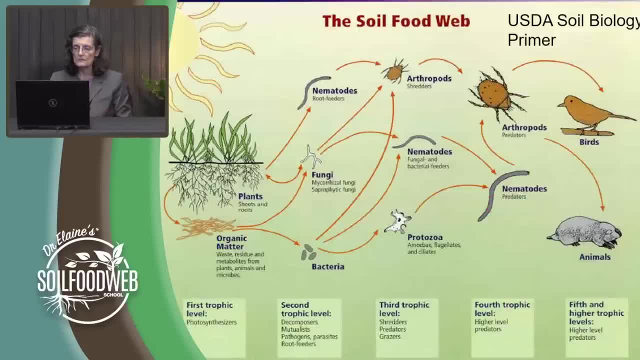 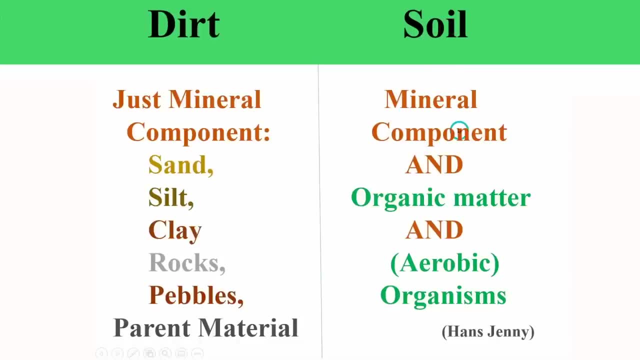 about how this below ground system works. So what's the difference? We've talked about soil, where that mineral component, the sand, the silt, the clay, where does sand, silt and clay come from? Well, it comes from the rocks, from the pebbles, from the gravel. 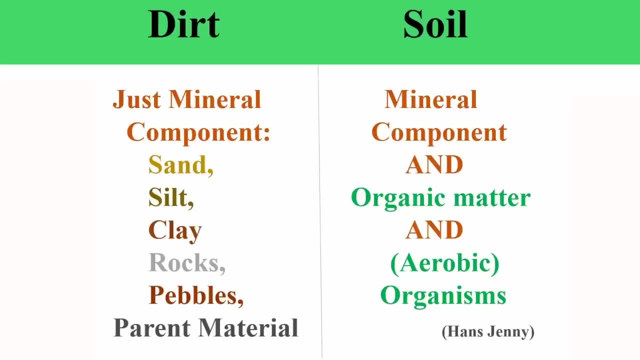 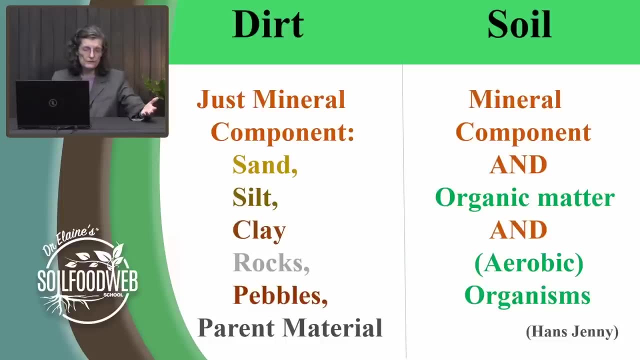 And how does that rock material get broken down and turned into those different size materials, the sand, the silt, clay and also the clay. I'm going to go over here to the dirt, because dirt is just the mineral component. It is just the sand, silt and clay. 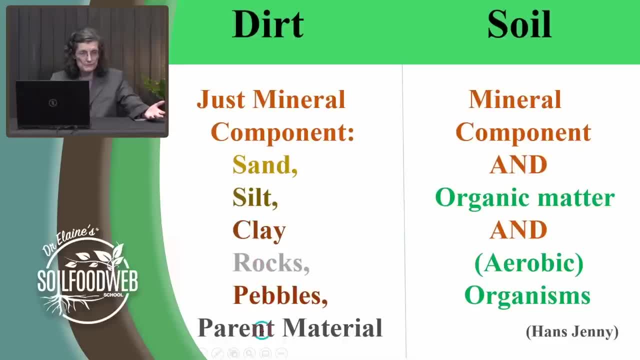 So as the rocks and the pebbles and the boulders and the parent material break down, what's released are those real small clay platelets and they bind together and cause those clay particles which are about the same size as bacteria, So about one micrometer diameter, one micrometer thick. 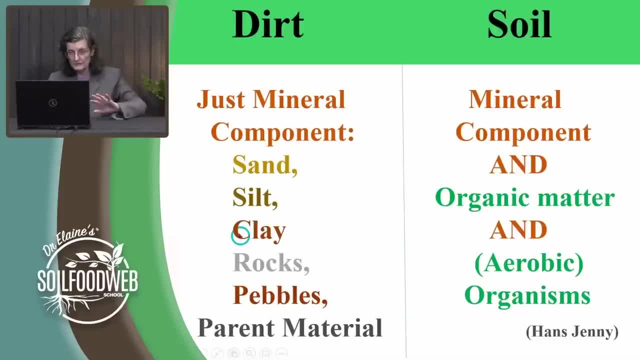 So they look very much like bacteria. You have to show you those differences between clays and bacteria so you can count those Bacteria reliably. Silt is quite a bit larger than clay, So silt is, you know, too small for you to see with your eyes. 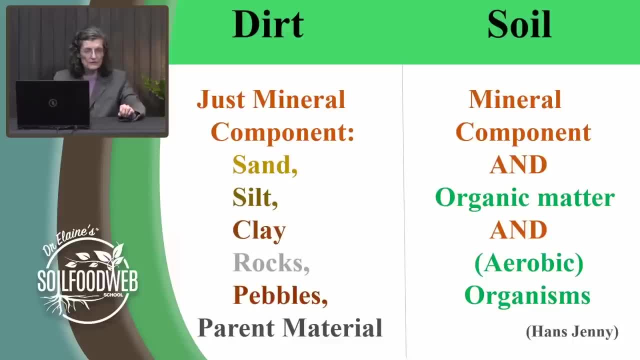 But you could. if you could see really finely, you could probably pick it up in forceps. They're the size the silt is the size of red blood cells, for example Sand. you can typically see sand with your eyes. 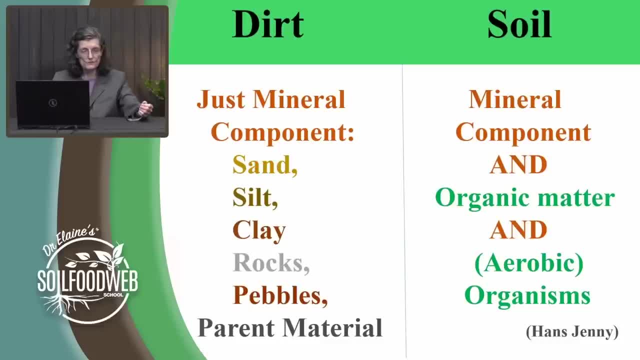 So you could definitely pick up sand particles with a pair of forceps or a pair of tweezers. All of these contain nutrients In the multi layers of the silica, in these compounds, glass sullae and, of course, in the rocks and pebbles and parent material. there is a lot of nutrient being held sequestered. 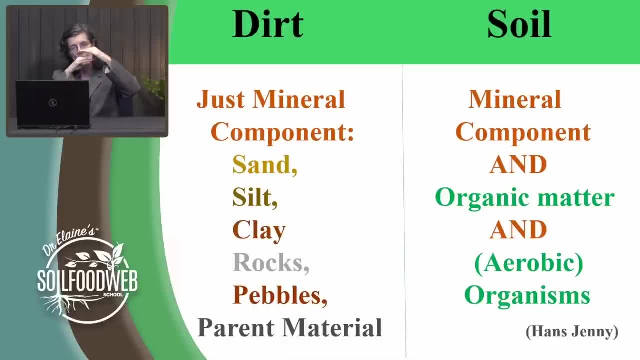 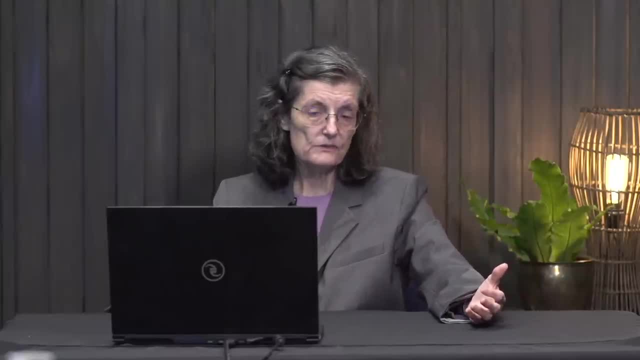 in that the layers of the silica, as I see it, spread in the soil, the materials. you have lots of nutrients. How is your plant going to get those nutrients out of the soil? or out of the sand, silt and clay? Well, not going to happen in dirt, because 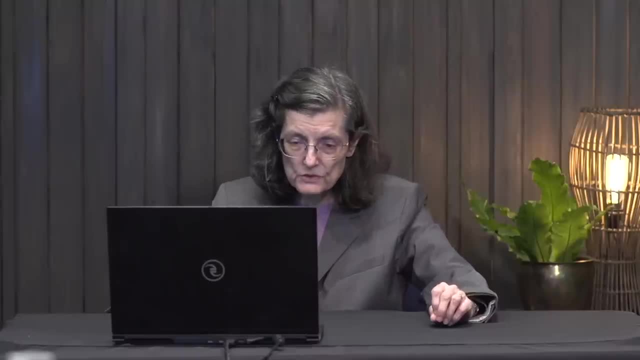 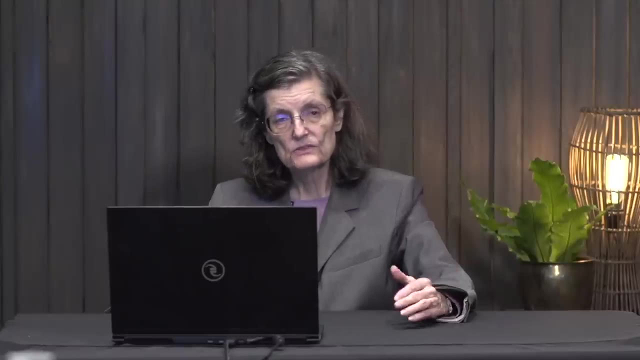 the organisms that do that work of pulling the nutrients, the mineral nutrients, out of these materials aren't present in dirt because there's no food to feed those organisms. We have to start getting organic matter back into this system for us to start to call it soil, So the mineral 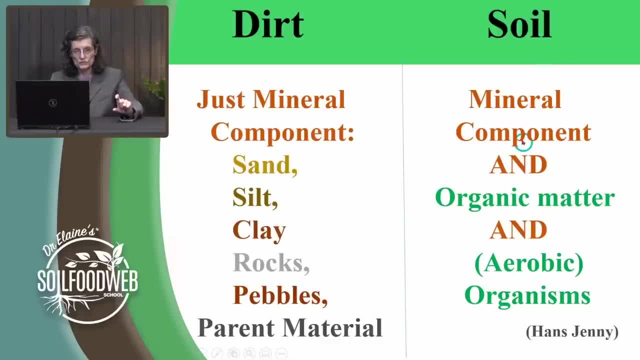 component: yes, sand, silt and clay. the texture Now, texture is not soil. Texture is a part of what soil is, but definitely Not the whole thing. So dirt sorry, not soil. So we have to have the mineral component and 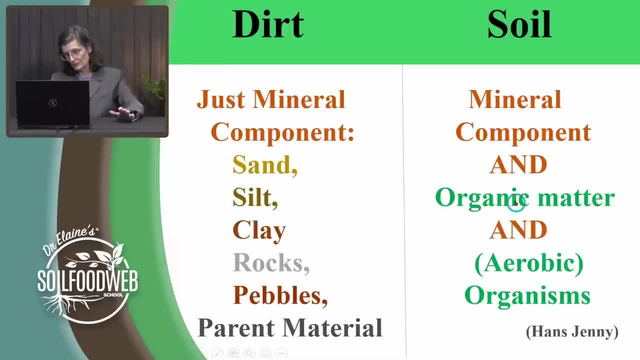 organic matter in order to feed the bacteria and fungi and have these bacteria and fungi perform their functions. And we were talking about those functions yesterday, the overarching principles that are supplied when you have these aerobic organisms present in the system. Now, this particular definition. 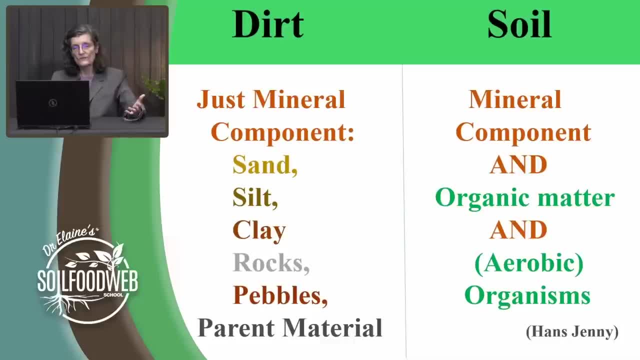 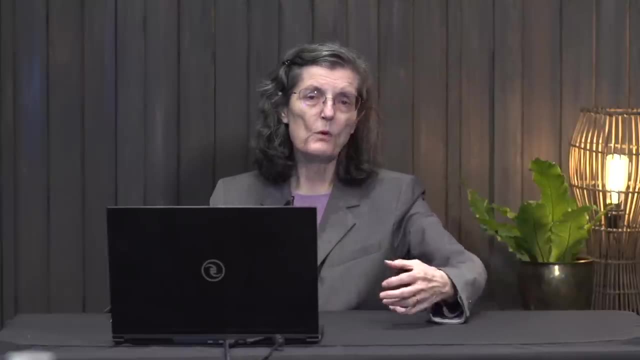 of soil comes from Hancieni, one of the fathers of soil science. He assumed that everybody understood that soil is aerobic, that soil has to have the air passageways and hallways, the pores, the structure to hold water, to allow oxygen to move into the soil. allow your organisms to move in there and, oh yeah, allow water to infiltrate and be held deeper down in the soil. So that's what we mean when we say building soil structure. We have to have adequate organic matter. But how much is enough? The minimum level to get the benefits of growing things in soil is 3% organic matter. 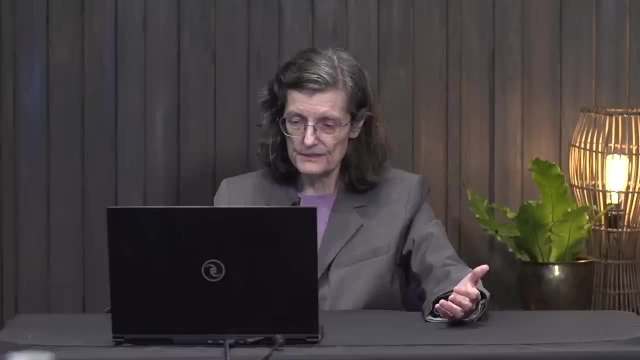 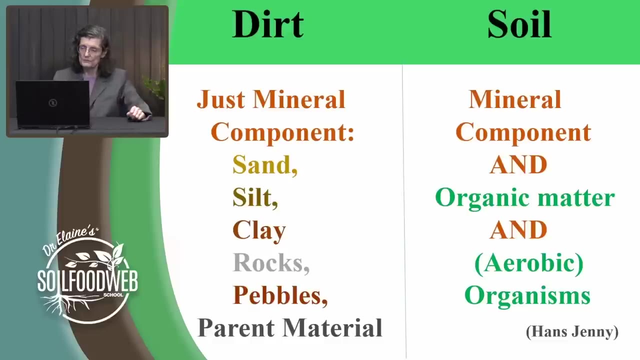 You have less than that and it's awfully hard to keep your organisms alive and active and functioning throughout that whole growth period. So we need the aerobic organisms, the organic matter and the mineral component in order to have this be soil. Should we have more than 3% organic matter? Absolutely. I don't know any plant material that is not benefited and life is made easier for you as a grower. 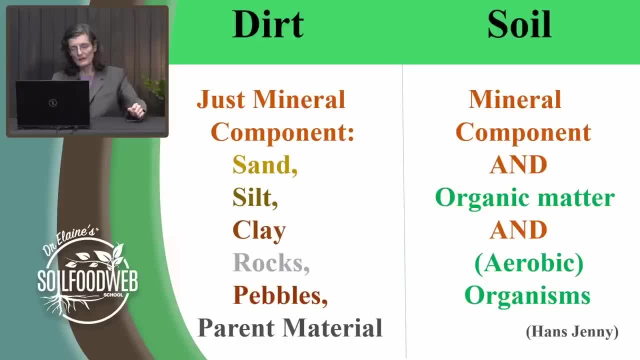 If you have higher organic matter in the system. So 5%, absolutely Keep going. 10%, 20,, 30. My favorite soil is made from the organic matter alone, with the aerobic organisms in there, Because when you think of organic matter, 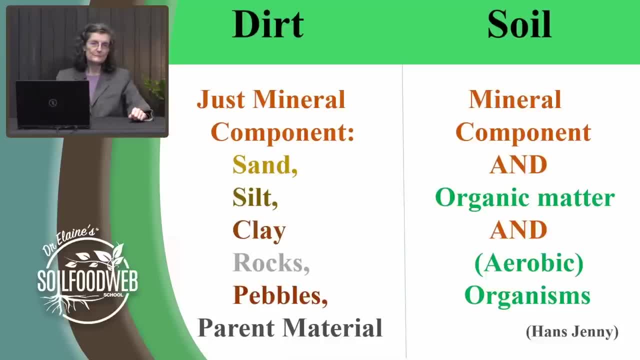 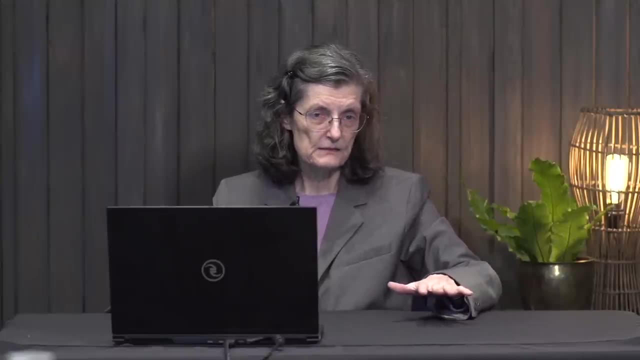 where did that organic matter originally come from? It's dead plant material? Are there any nutrients in that dead plant material? Well, of course there is. It was a plant once upon a time. That means that plant tissue had to have all the nutrients present in it that any plant requires. 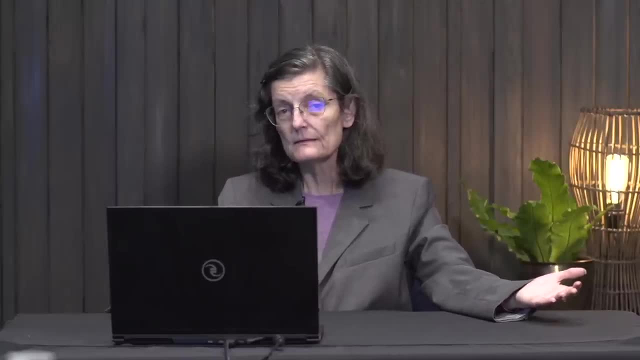 in order to be able to perform the functions of being a plant. So of course, there are nutrients in the organic matter. I know people will say, oh, but there's so much carbon? Well, not any more than a plant, And these microorganisms love to grow. 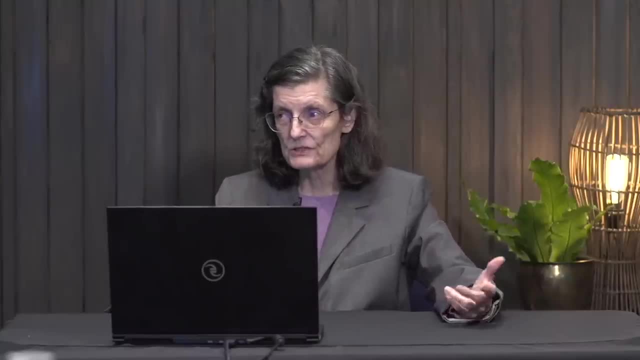 On the surfaces of your plant material, protecting your plant against diseases and pests and problem organisms. So of course it's got the nutrients, Your plant material residues on the surface of the soil, the dead root systems that after that plant can't make it anymore, that root system. is going to become organic matter as well- The aerobic organisms. they need to be around, And if you have killed all of them on your property, you're going to have to go out and find some more someplace and either buy really good compost or start. 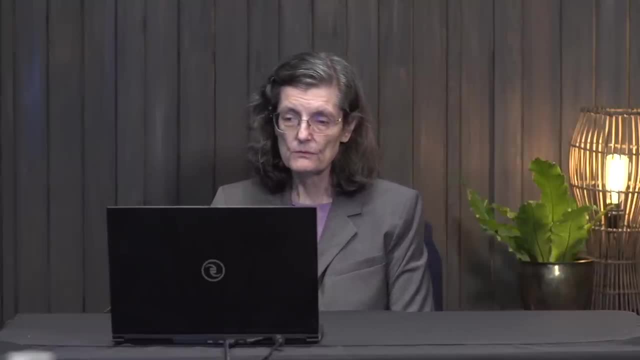 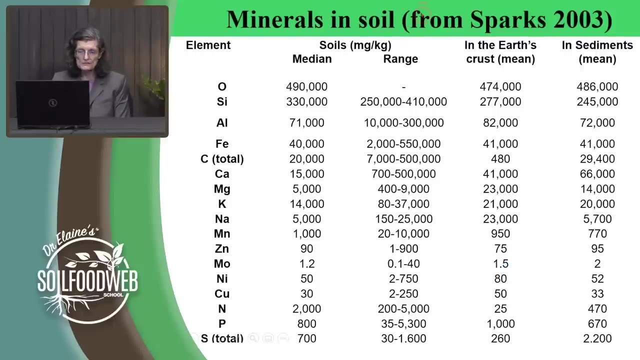 making it yourself if none's available. So when we look at the nutrients in soil- and now this is an excerpt from Sparks 2003.. So it's a little bit different from what he presented- Removed some extraneous material Didn't need in. here It's about we're looking at the elements, So oxygen, silica, aluminum, iron. 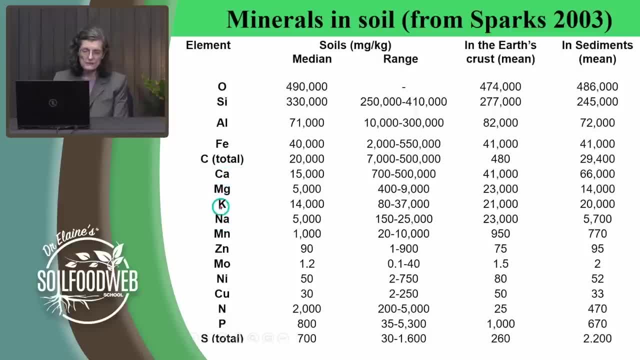 you know, here's calcium, magnesium, sodium, manganese, zinc, Here's copper, Here's nitrogen, Here's phosphorus And here's sulfur. So when we look at the total, so this soil, the concentration of these elements or minerals in your soil and the median, the 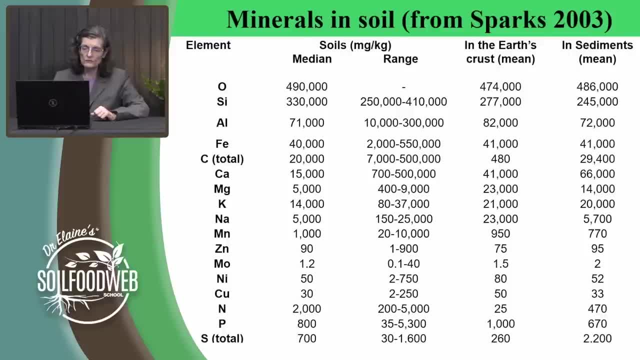 on average in general value for these organisms from soils from all over the planet. you can see there is no nutrient that we lack in soil. How much calcium does your plant require, for example? Well, what's in one kilogram of your soil is fifteen thousand. 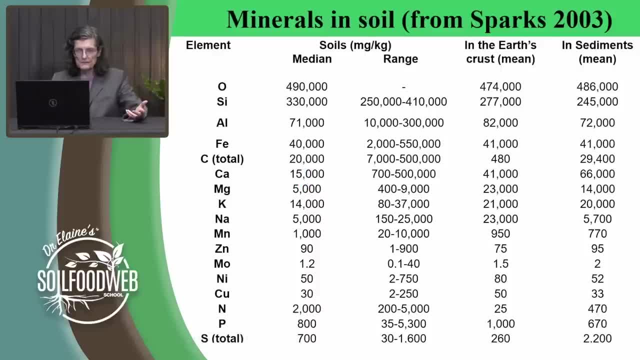 milligrams of calcium. This would last your plant if it could just suck that material out of the soil through the whole entire growing season. This 15,000 milligrams per kilogram of calcium would probably last you for something like 70 years, And remember every second of every day. 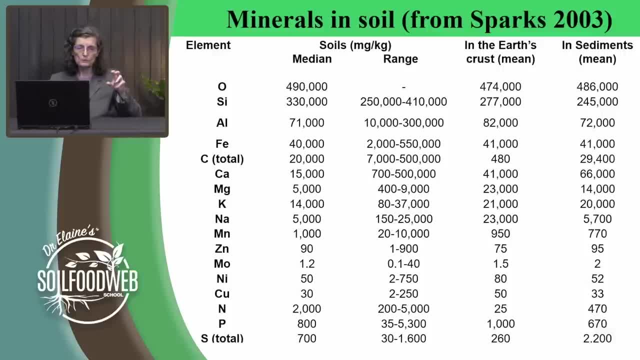 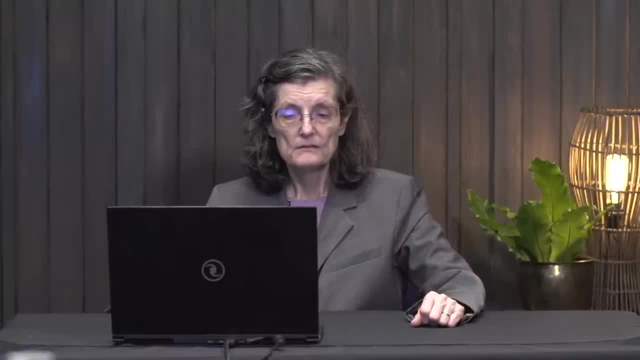 the rocks, the pebbles, the boulders, the apparent material boulders are all being broken down every day by bacteria and fungi. So the weathering of rocks is not the most important thing. It is the action of the organic acids, the materials that bacteria and fungi make. 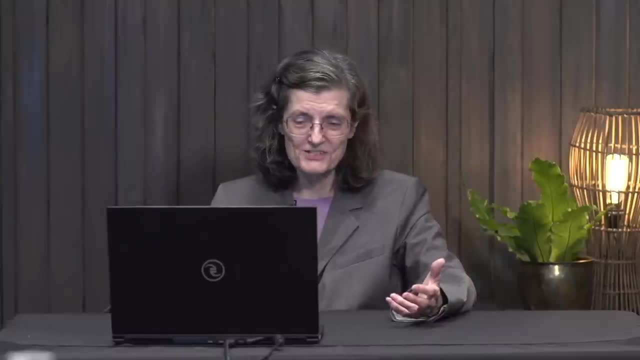 that causes these larger chunks of rock to break down eventually. So until the day you run out of sand, soil, clay, rocks, pebbles, apparent material and boulders, you don't have to worry about nutrients: It's already in your soil. There is no soil on this. 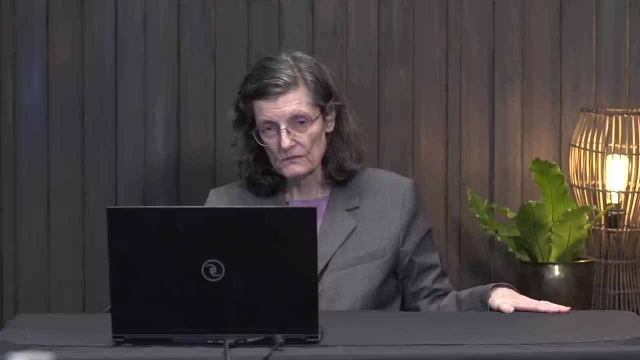 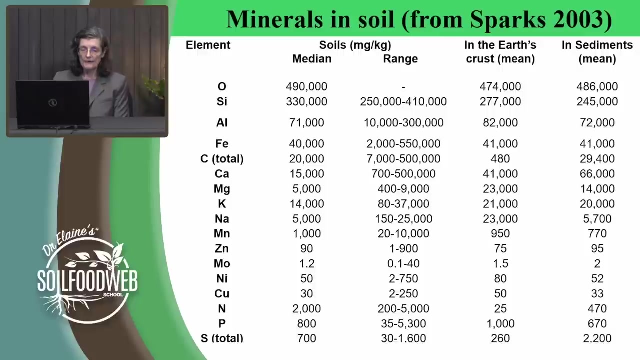 planet that lacks the nutrients to grow plants. So why are we putting inorganic fertilizers out? Well, if you kill the organisms in your soil, then you have to use those chemicals. So we have the nutrients that we need. We don't have to be worried about that. We just have to be. 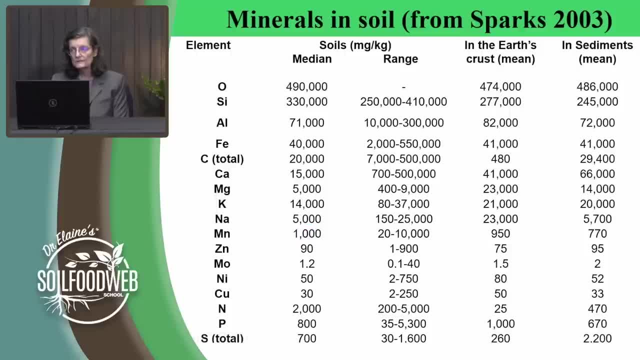 worried about whether we have the biology to get things started Now. so after 70 years, you know, if you didn't have more sand, soil and clay joining the fray, you might have to start worrying. So what else holds nutrients? Yeah, organic matter. So let's count on both of them. So 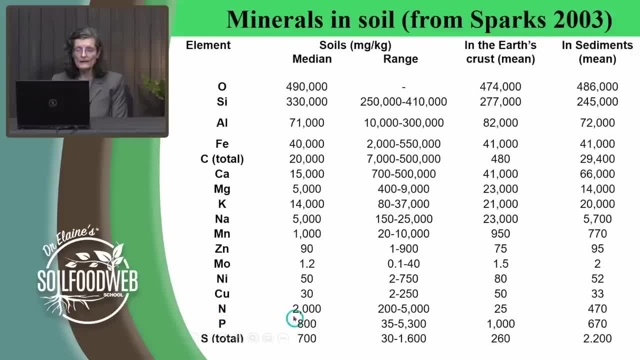 look down Here at nitrogen: on average in general 2,000 milligrams per kilogram. That's way more than any crop requires, And we've got something on the order of you know 50, maybe well, depends on. 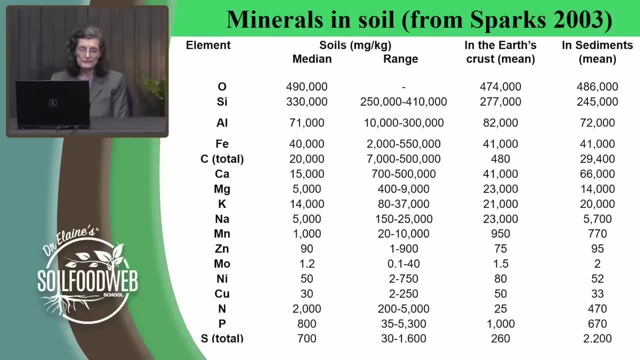 exactly what's going on. But you've got plenty of nitrogen, You've got plenty of phosphorus, You've got plenty of sulfur, So you don't need those inorganic fertilizers And we're going to be putting a whole lot more. 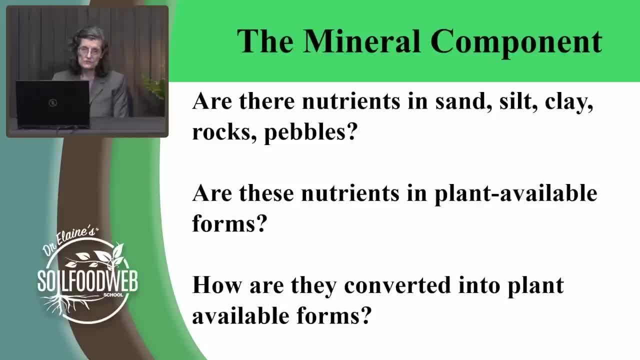 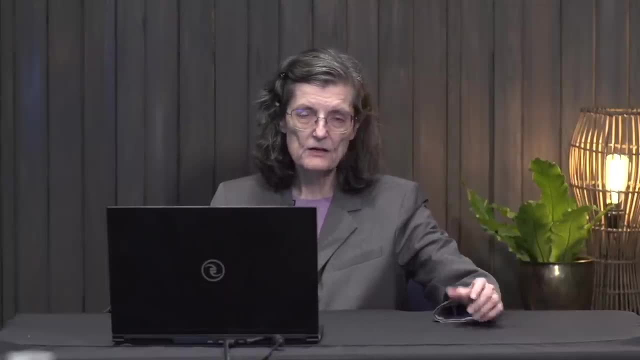 of the organic material into the soil, So nutrients will come from the organic matter as well. If we have those low-growing cover plants, the ground cover, those plants will make certain all this nutrient cycling is happening. We get the root systems of those low-growing plants. covered with the mycorrhizal fungi that your plant requires. Then the instant you put the seed into the soil and the seed starts germinating, it's going to be connected into the below-ground network that the mycorrhizal fungi establish Every single plant in. 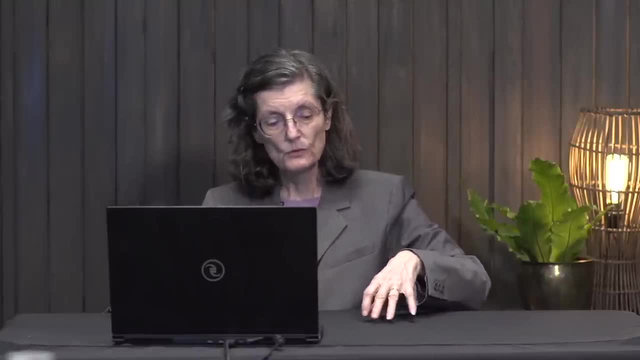 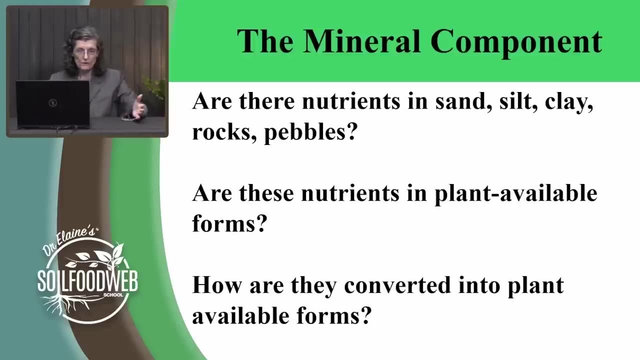 that field that can become mycorrhizal will be healthy, And that's what we want to make certain is happening for all the crops that you're growing. So how are they? how are these nutrients in the soil? How do you make them plant-available forms? How do you make them plant-available? 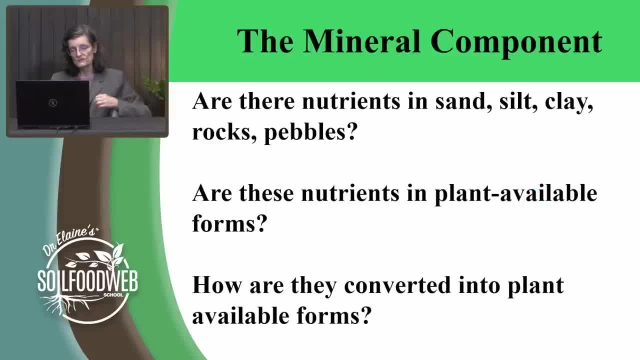 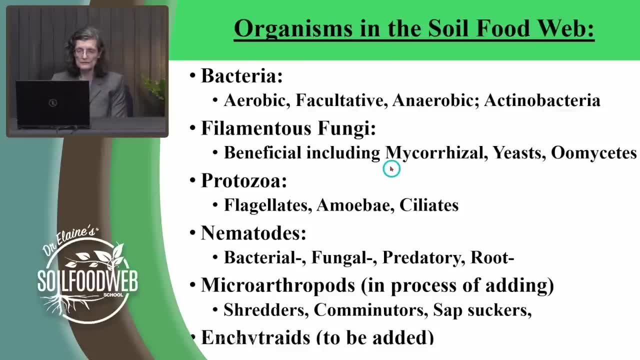 How does that conversion happen? And we talked about that yesterday, so I don't think we have to go over it. So again, all of the organisms in the soil. we've got to continue to think about those, And so I'm going to go through pictures. How do you identify some of these? Just to start giving. 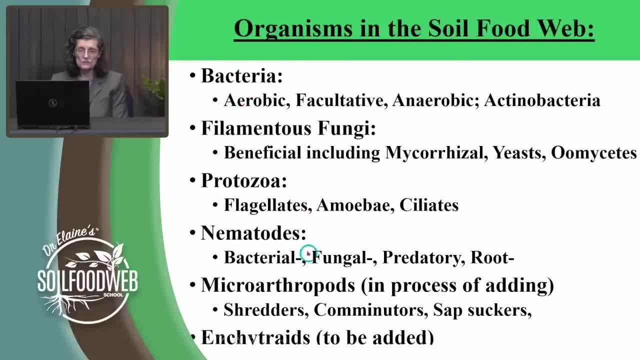 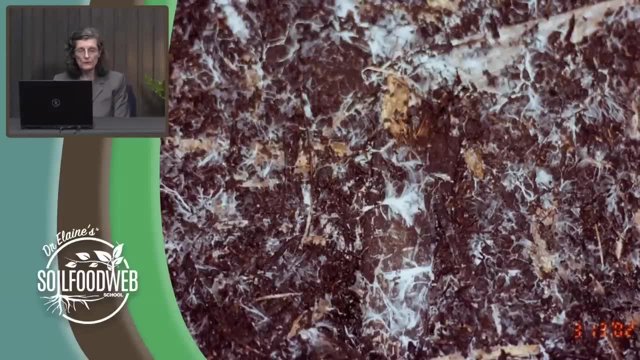 you a clue of the kinds of things you're going to be introduced to, in order that you can be doing this work for yourself. You can do this work for your neighbors, for your friends as well, And so we train people how to identify: is this a good guy fungus or is this a bad guy fungus? 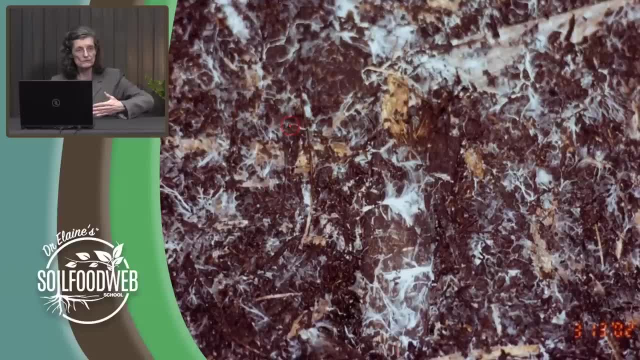 Well, just by looking at a block of this soil, just cut that, cut it out using a shovel and kind of cleaned up the surface here so you could see clearly where that white fungal hyphae is growing in here. Yeah, it's kind of lined up with the woody material. 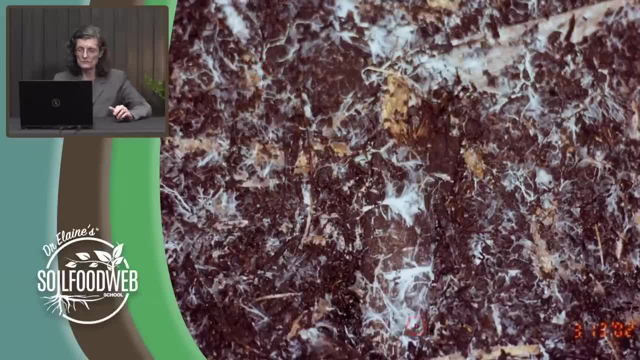 with the, you know, broken up parts of woody materials that were added into this block of material. You can see where that woody material has been broken down and it looks like soil. good structure, lots of airways and passageways in here, so excellent structure You can take. 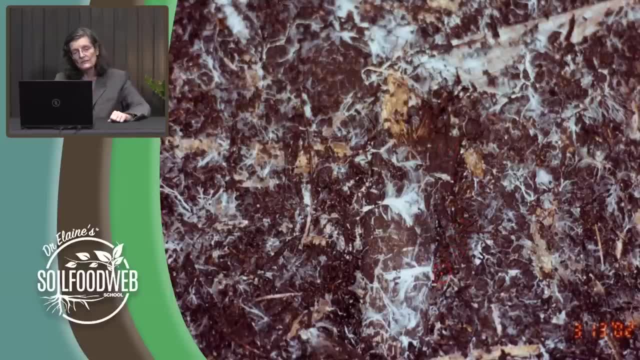 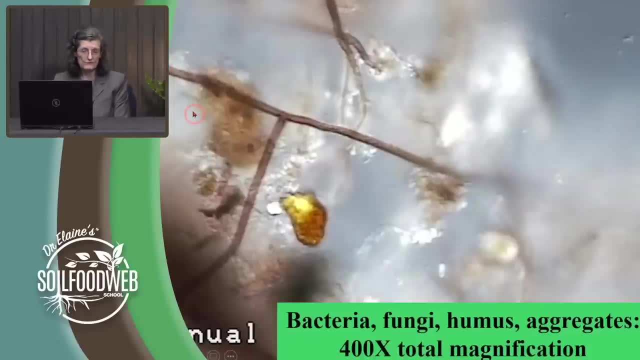 out and look at what the biology is in that material. So when we're looking at something like this, we will find fungi. Of course you're going to find fungi because look at the massive amount of fungal biomass you have in this material. So fungal hyphae: we teach you the characteristics of fungal hyphae uniform. 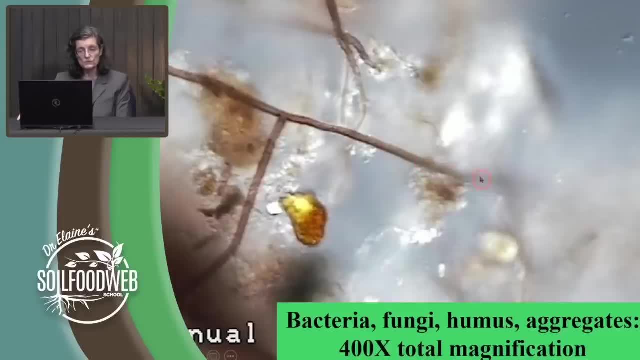 diameter all the way along the strand. You may have changes in diameter when it branches, but you know, there we are some more of that particular fungus. You can see septa. these are cross walls, but these are adventitious septa. They only 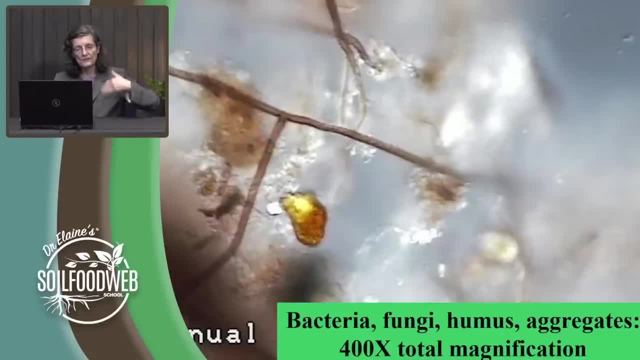 happen on occasion. They are not uniform. So in general those fungi and that have uniform distances between their septa are more likely to be beneficial. but you know, this guy is probably still beneficial even though it lacks one of those characteristics. Well, what are the other characteristics? Color, 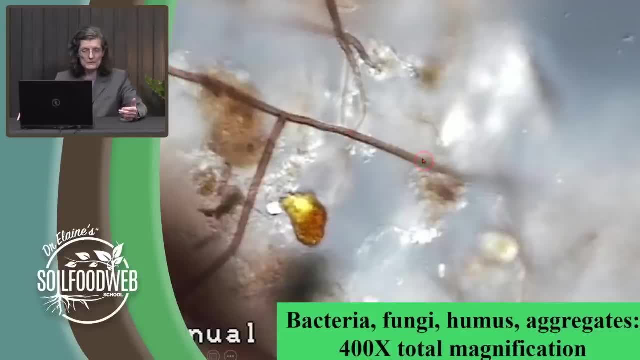 Typically, color means the darker the color means the more likelihood that this is going to be a beneficial fungus. Now look out. we have a few disease causing organisms in the wild. So we have a lot of fungal hyphae in this group of fungi. but those 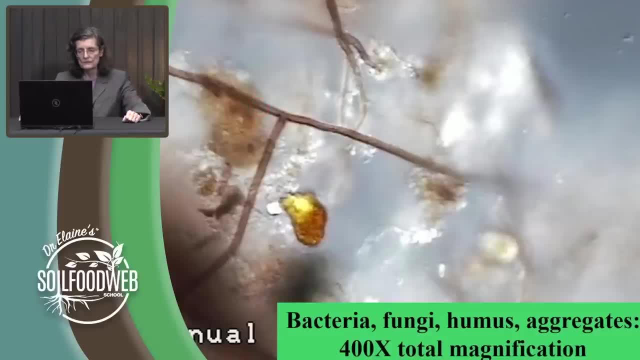 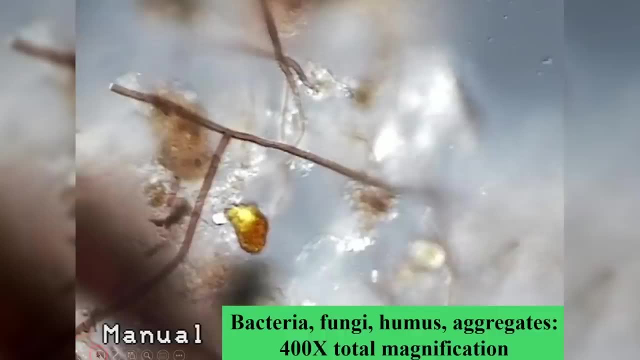 distinguishing characteristics can very easily be given to you. So we have another strand of hyphae. down here in the bottom left hand corner You can see a slightly narrower diameter, so still wider than three micrometers. Brown tannish. so it's, it's um, it is colored, So most likely this is a beneficial fungus. I can't. 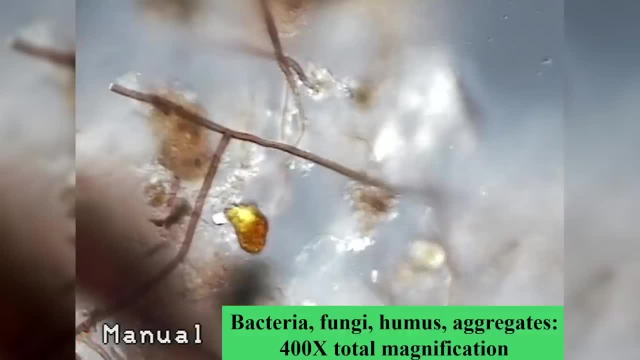 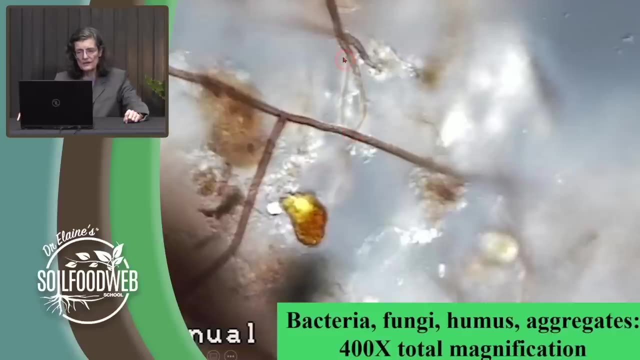 see whether it has septa in a row or whether it's adventitious again. These individuals right here, these strands, are they the same fungal hyphae as this, Or is it a different species? Well, it doesn't look like. it's even uniform. 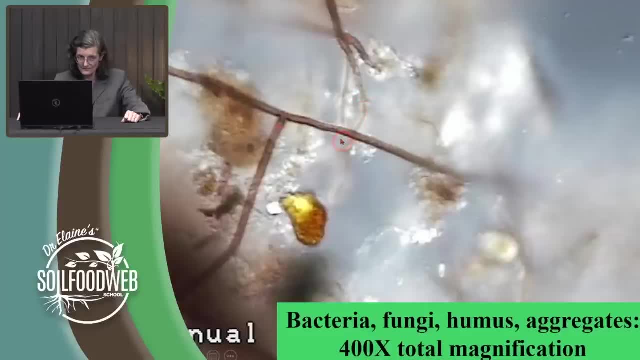 diameter all the way along, but it is If you use your focus knob and you've got a focus all the way along. bring the edges into nice sharp focus like this, and you'll get a nice sharp focus. So this is a fungal hyphae that's not quite as good as the other ones, but it's. 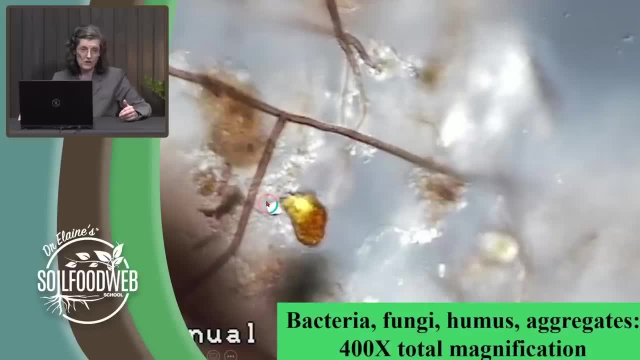 a fungal hyphae that's not quite as good as the other ones. So we have a lot of fungal hyphae that look like they are right here In order to be able to tell whether it's uniform diameter all the way along. So we have another fungal hyphae right here. 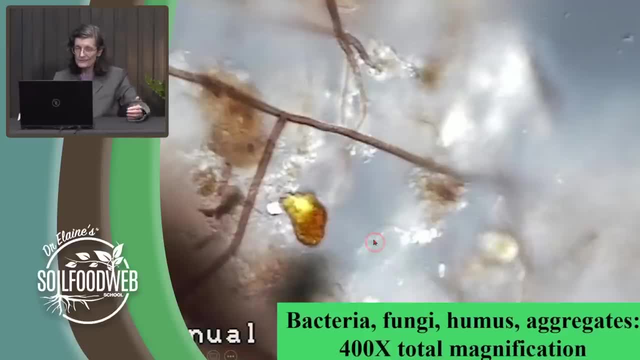 You can see. it's clear, it's colorless. That's not quite such as good. so much of a good indicator. but look at the wide diameter. So wide diameter is better, colored is better. but when you're mixing and matching some of these characteristics, 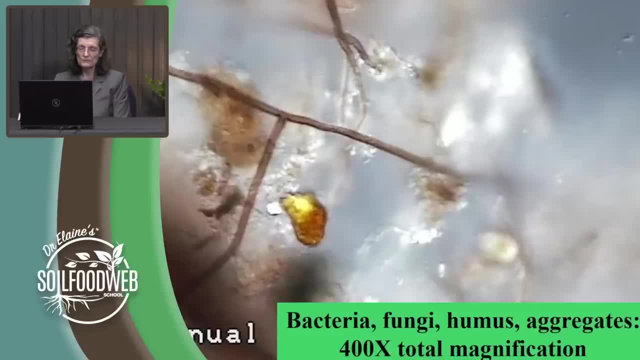 it still can be beneficial. So the wide diameter beats the clear or colorless condition. So we have testate amoeba way out of focus right here. There's lots of other creatures, lots of bacteria in this picture. There's several hundred thousand bacteria in this area right alone. it's hard to count, So we would 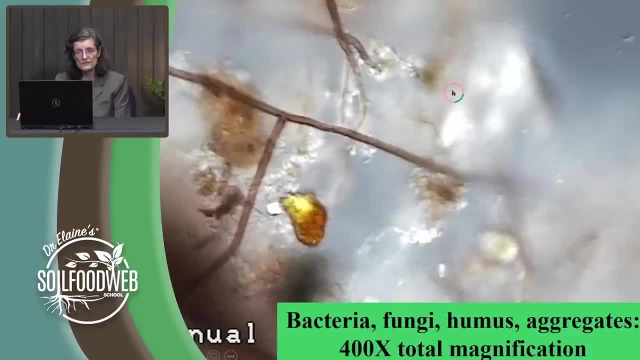 choose to dilute more when we get to the stage of trying to count the bacteria in this sample. It's just so chock-full of really good things that you know this is going to make a great potting mix for your plants. They are 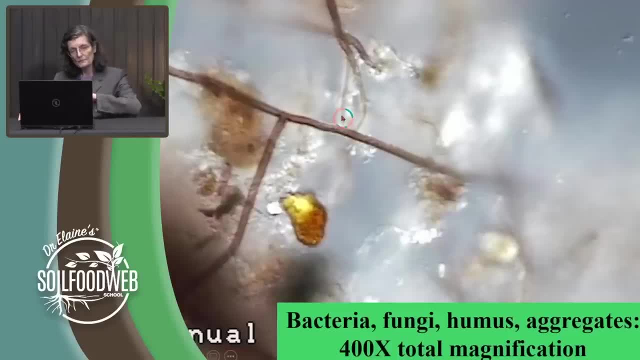 going to adore this. The biggest problem with a lot of organic matter in pots or in your in your soil is that so many people have the overwhelming urge to overwater This kind of organic matter. this really well-structured material has a huge water. 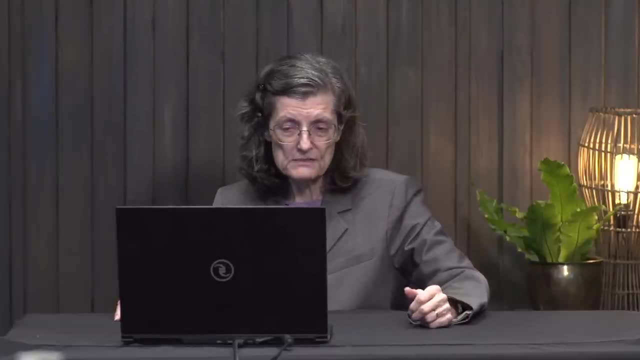 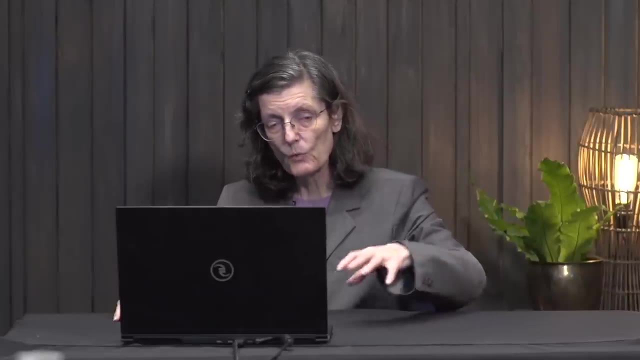 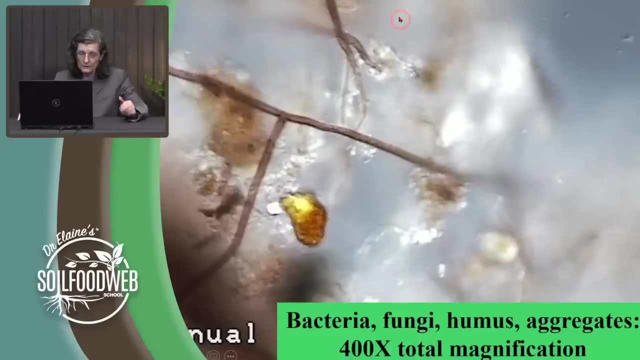 holding capacity. So it can be holding something like 10 to 20 times its weight in water. That's how well-structured this material is. So there is a disease-causing fungus in here, and the way we figured that out is it's very narrow. 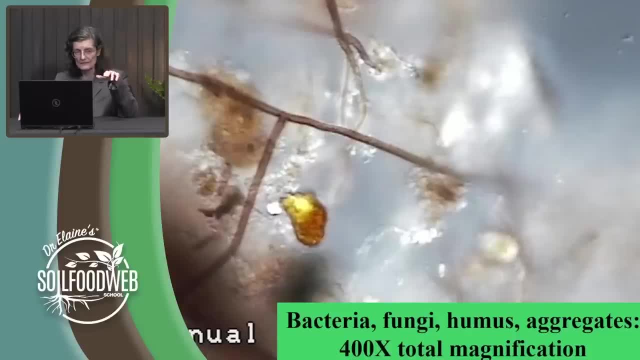 diameter. it's clear, colorless. it doesn't have any septa. you want to worry about those guys? So there's an example right here of a fungal hypha that is probably a pathogen. We plated this material out in a petri dish because we 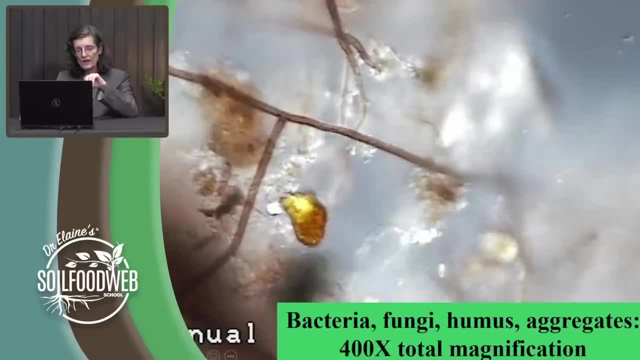 knew that none of these other fungi even had a chance to be able to grow on that petri dish. Those conditions are completely impossible, wrong, completely the opposite of what is needed to grow these fungi. Fungi are obligate aerobes for the most part. The filamentous fungi are going to be. 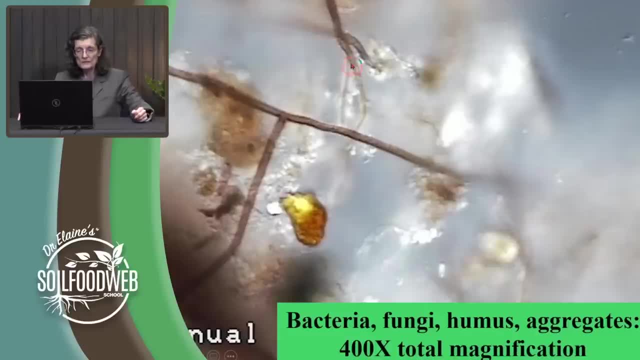 obligate aerobes. This particular fungus is Pythium. It is one of those disease causing fungi, and so when you put it on a plate with a lot of the foods that it requires, it starts growing very, very rapidly. and because you've put a lid on 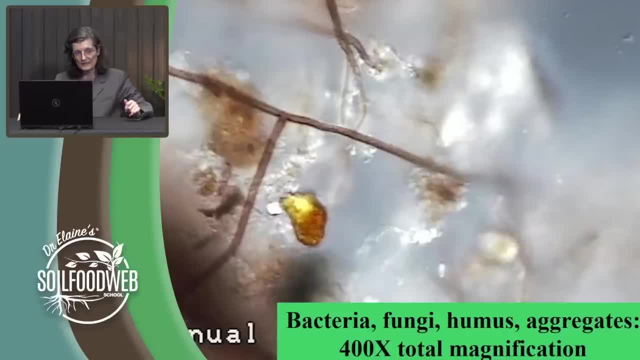 that plate. oxygen can't get into the plate and this fungus is going to have a grand old time growing and taking over your whole entire plate. So you start talking to somebody who does this kind of testing and they show you the Petri dish with that massive white, fuzzy, wuzzy stuff inside and they go: oh you look at. 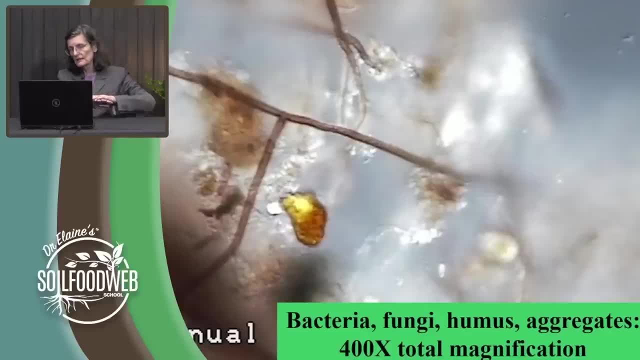 all of the disease causing fungus you've got. This is just going to take out all of your plants. You better get out there now and put a fungicide to prevent the growth of these fungi. And what is it that you actually kill? It's not the disease-causing fungus. It's all the good guys, So this is a self-fulfilling prophecy that is absolutely and completely and totally wrong. If you had not applied the fungicide and not killed all these beneficial organisms, that Pythium would never have had a chance. I have potted plants in this kind of soil over and. over and, over and over again and I have never lost any of those plants to the Pythium taken over. because the Pythium is going to be out-competed, It's going to be consumed by one of the beneficial organisms and it's going to be consumed by one of the beneficial organisms. 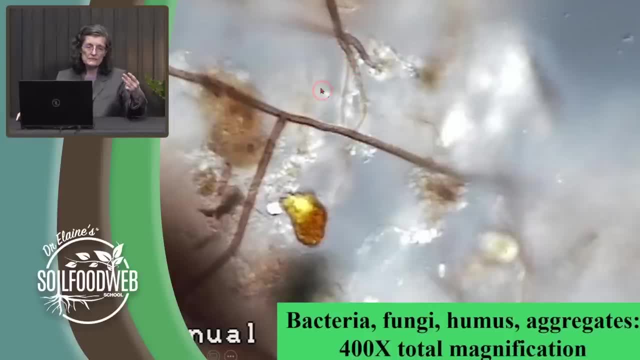 predators in the system and it's going to be attacked by and dealt with by, inhibitory compounds made by some of these organisms, But in the soil antibiotics. these inhibitory compounds are not released out into the whole soil. They don't cause mass sterilization. Those inhibitory compounds are only 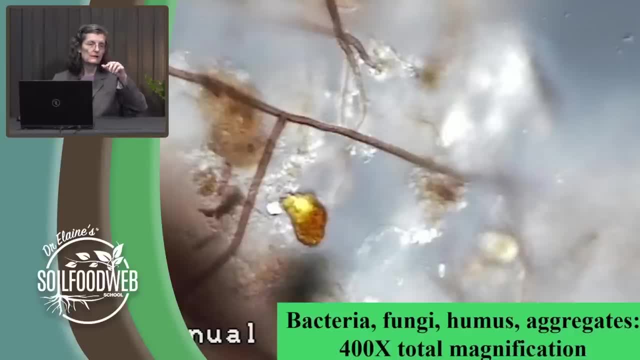 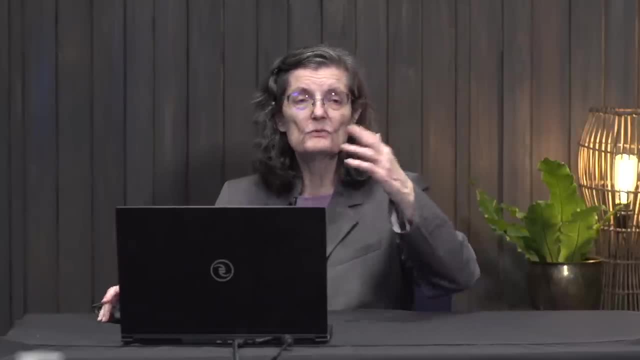 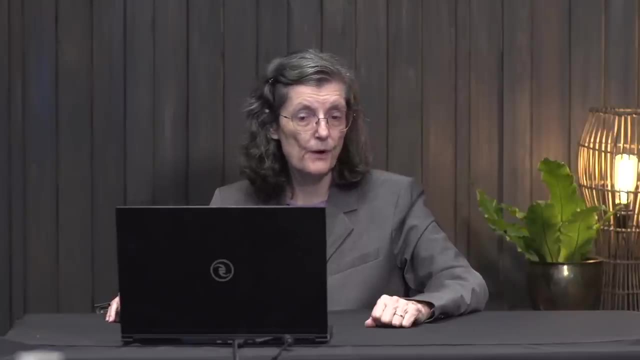 released right around the body, But it doesn't harm the whole body. So you don't have to worry about the bacteria or those fungi that are there. So you'll be able to reduce the population. but you need all those other interactions to really control something. 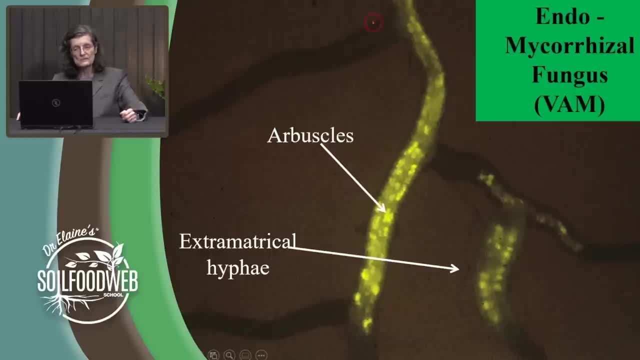 and prevent that Pythium from being able to grow. So let's keep going. This is a root system of an onion and you can see the auto fluorescent arbuscules formed. The endomycorrhizal fungus, or more commonly has been called vesicular arbuscular mycorrhizal fungi. so VAM. 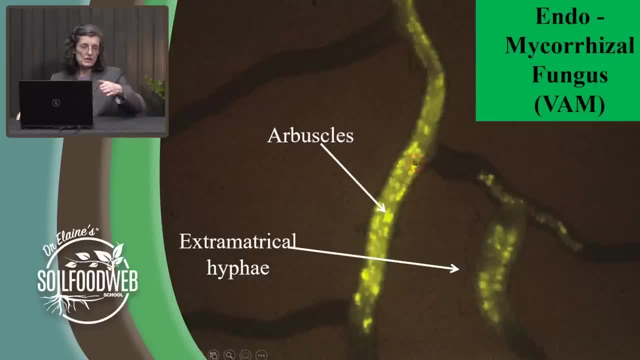 The arbuscular is where the exchange between the plant and the fungus occurs, So the plant is happily making all kinds of photosynthate. The photosynthate comes down into the root system, where it's colonized by the mycorrhizal fungi. 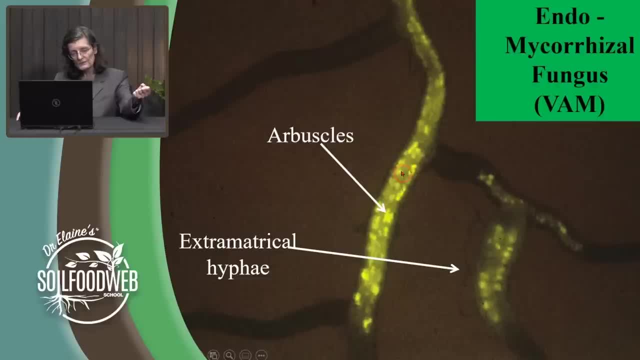 The plant gives that mycorrhizal fungus some food, along with a message basically published in biochemistry given a message that the plant needs whatever the plant needs. So let's say it's calcium. So the plant is telling the fungus. 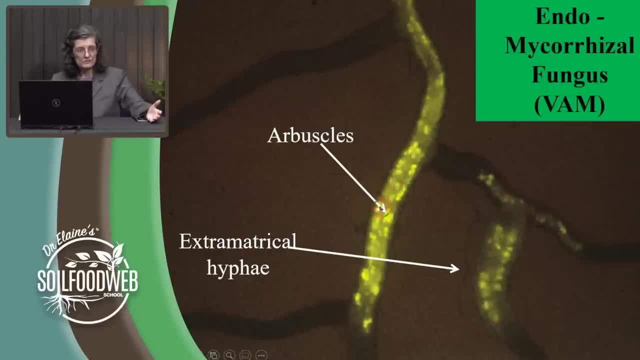 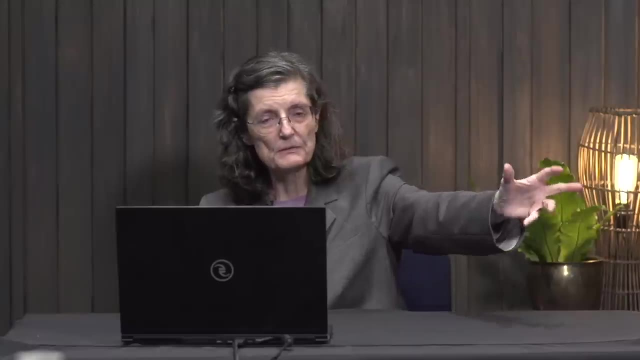 to go find some calcium, and the fungus is more than happy to do that. So you can see some of the hyphae out here where that fungal hypha is going to grow out into the soil way over here and find some calcium. 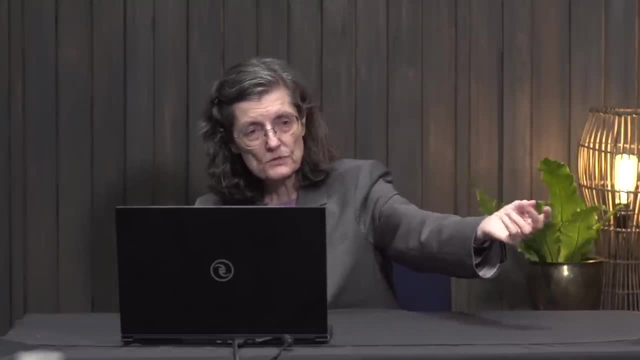 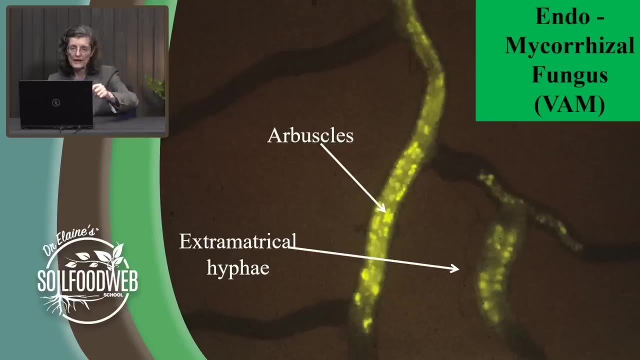 use its enzymes to pull that calcium out of the sand, silt, clay, rocks, pebbles out of the organic matter and translocate that back to that arbuscular And the fungus now says, hey, plant, I've got your calcium. 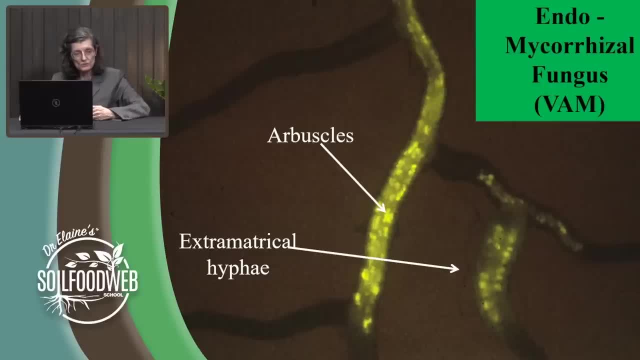 I'll trade you that for some more of those great sugars you were feeding me, or proteins, or amino acids, And so both organisms benefit. And, of course, then what's the plant going to do? Well, if you want more of this food, then you have to go find me some water, and I need some phosphorus. 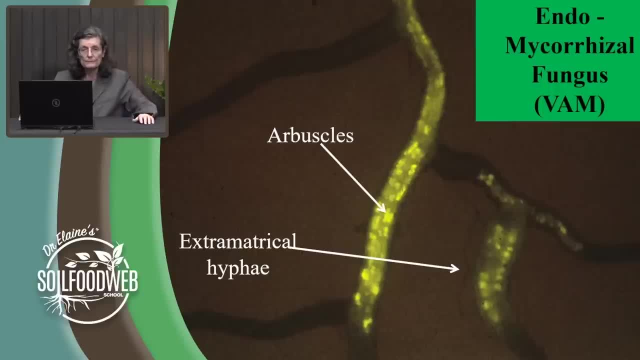 And gee, while you're out there, I want a little bit of sodium. And the fungus says, yeah, no problem, There was plenty of that out there. And so back through the hyphae goes the message. here's what the plant wants. 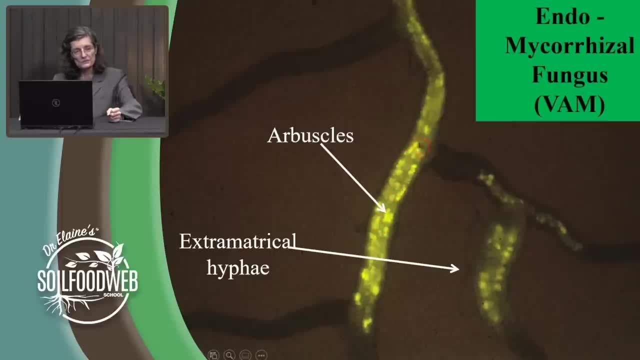 transport it to the plant. here and through the arbuscular, the exchange occurs. Why the vesicular arbuscular mycorrhizal fungus makes that autofluorescent compound, nobody really knows. No one's looked at the metabolism of endomyelitis. 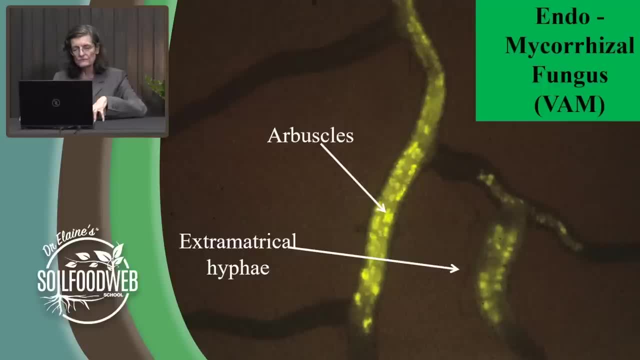 it's just a little bit of a. There are many different types of fungi, but this is the most common one. It's called a microysyl plant species or fungi to figure out why, But this only occurs when the plant and the fungus are interacting together, So it's these interactions that are really important for us. Can you estimate how much of this root system is actually colonized by the mycorrhizal fungi in this picture? So if you add up all of the places that are dark- no fluorescence- and you add up all of the places that are dark- no fluorescence- and you add up all of the places that are dark- no fluorescence, that's a lot of different things. 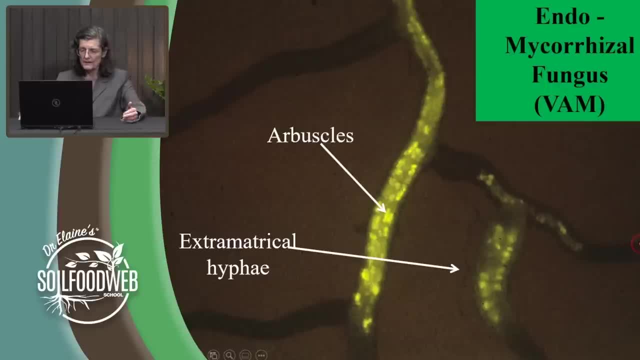 there's another little patch. there's another little patch that's not fluorescing, another little one there. and now compare those areas that are colonized by the mycorrhizal fungus. what's the percentage? now you can get this. you know, you can have a little ruler that you can use in your eyepiece. 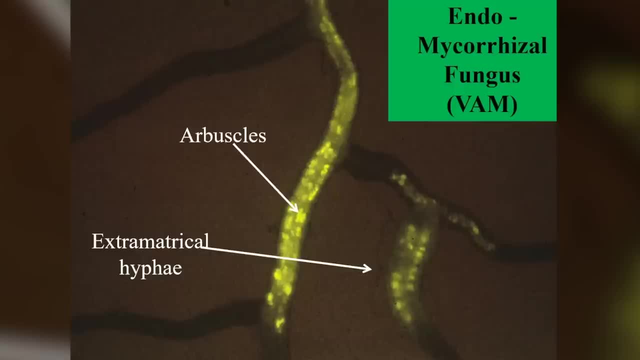 and and so you can get a fairly good idea of how much of the root system is colonized and how much isn't. so when I look at this amount that's colonized, I would say that there's about 40 percent of the total that is colonized by the. 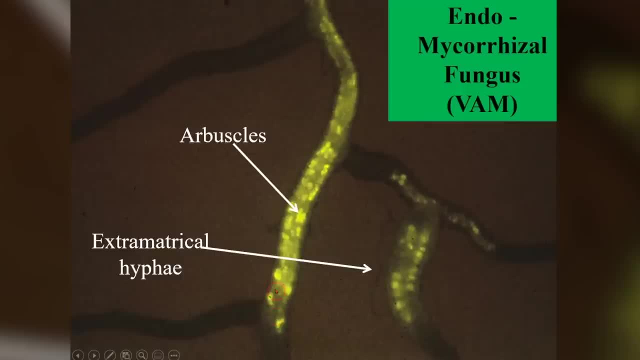 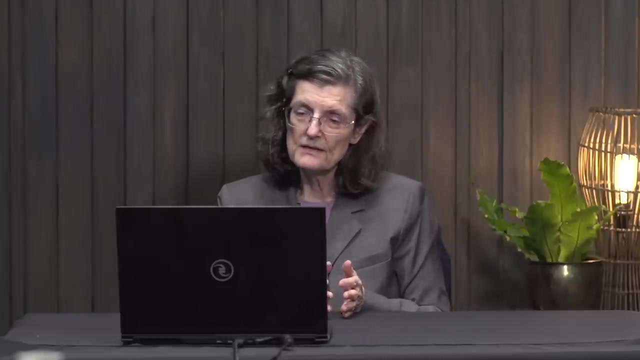 mycorrhizal fungi. we know and work that was done by folks at Colorado State University, John Moore. they've showed that as long as you have 12 percent, more than 12 percent, of the root system colonized by the mycorrhizal fungi that you will be receiving, your plant will be. receiving benefit from being colonized by that mycorrhizal fungus. but you know, can you get more? yeah, if you can get your root system colonized 40%, then you will get all of the benefits that that mycorrhizal fungus can give. obviously, they're pulling nutrients from the soil and bringing them to the plants of. the plant will grow better, so the mycorrhizal fungus will grow better. we also know that the mycorrhizal fungi will translocate water, and so in a drought period, you need to have your. plants colonized by the mycorrhizal fungi so that the fungi can grow the root, grow the fungal hyphae down 10, 20, 30 more feet. we know that the hyphae of mycorrhizal fungi can extend out for 300 yards. that research has been done and published. there's others saying the length of a football field. so how deep into the soil can the mycorrhizal fungi go? well, it's going to increase the amount of water that your plant can obtain in a dry, droughty summer period. so your plant survives. it produces yield. 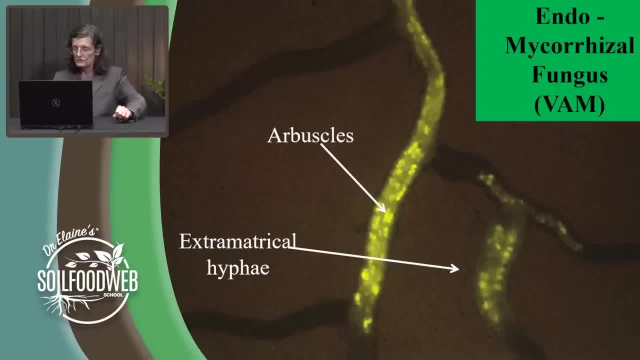 and you as a grower are going to have some money in the bank, so we really want these mycorrhizal fungi in the proper plants. ectomycorrhizal fungi are colonized, colonize the root systems of evergreens, conifers, the endo mycorrhizal fungi. 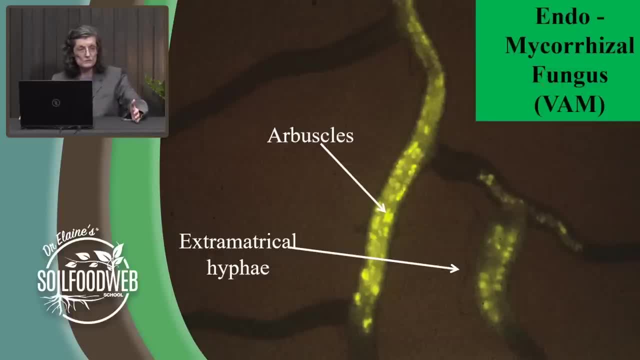 colonize everything from through the deciduous trees- this is, deciduous shrubs- through the highly productive grasses, the tomatoes and the tomatoes and the tomatoes, the solanaceae, through the onions, the garlics. most of our veggie materials require mycorrhizal colonization. but then that set of plant. 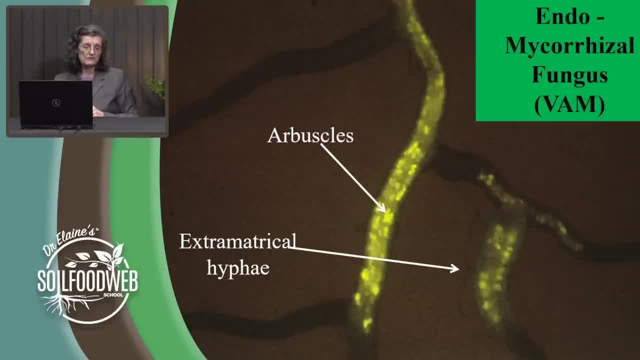 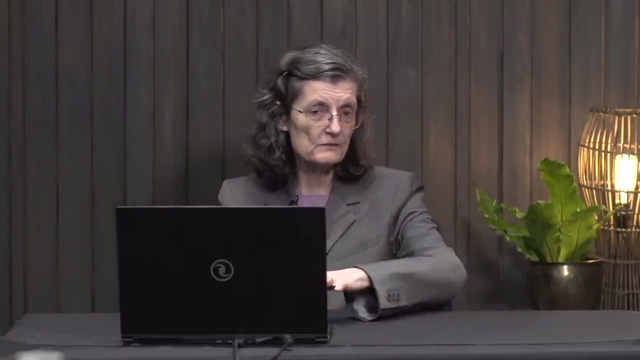 species that should not become colonized by mycorrhizal fungi: the coal, the kale crops, you know things like broccoli, cauliflower mustards. so as long as you're paying attention, you can make sure that your low-growing ground cover has the right kind of mycorrhizal fungus in the soil moving. 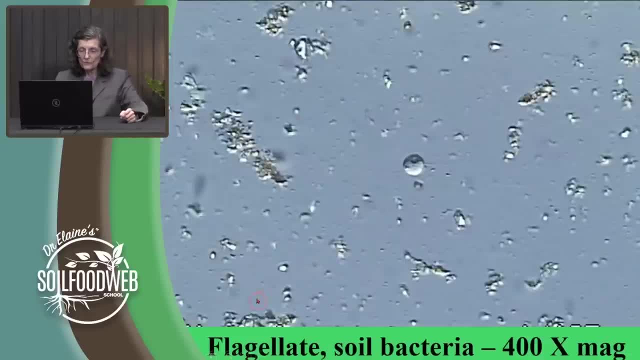 on when we're looking in here for a flagellate. it's really easy to figure him out because he's larger- my significant amount- than any of the bacteria. there's a flagellum right here and you do want to be looking for those little flagella. 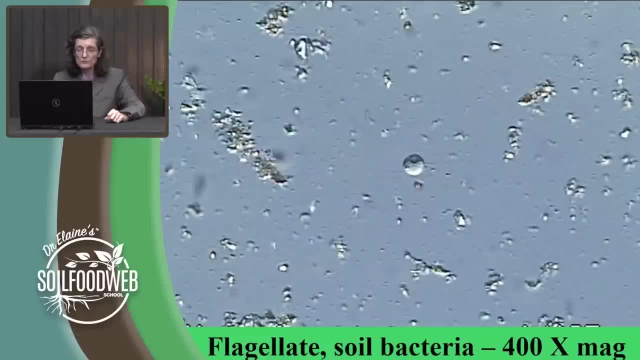 wiggling around in the soil, pushing the flagellate through the soil, and then you see the other fungal, the other flagellate. when you see the other flagellum of this flagellate- and that's right here, it is wrapped around the body. 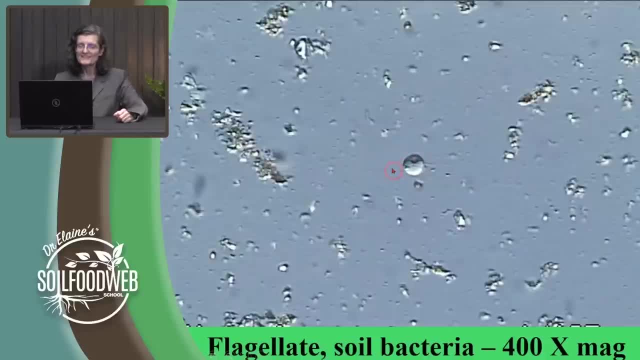 of this flagellate, and so, as this flagellate is moving through the soil, pushing along, this flagellate will bumble on one side. he'll be pulled to a one side because of this front flagellum being wrapped around the body, and so we. 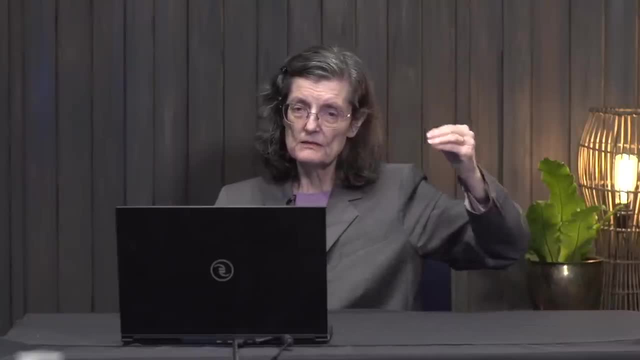 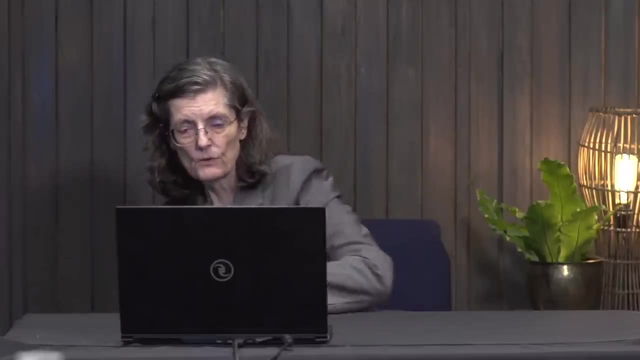 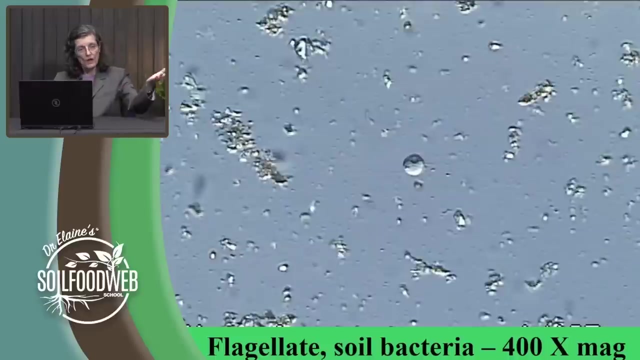 use this characteristic of the flagellate going through the, through the soil solution, and it does a sidewards tumble and then again sidewards tumble. so we're looking for that kind of distinctive motility and then you know that that's a flagellate, not just a small ciliate. 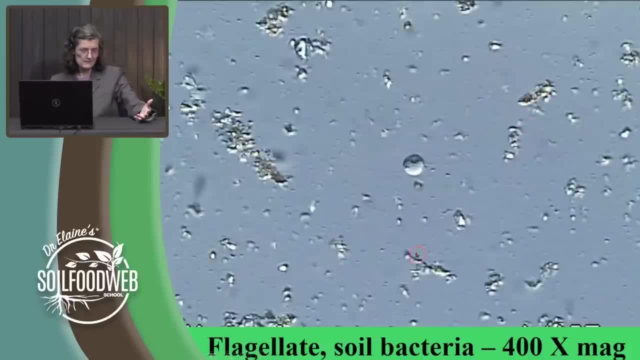 and I look at this particular picture. this is got me worried because, looking at how poor structure in the aggregates that the bacteria are building, this is not good. this is not a healthy soil. despite the fact that we are seeing a good guy, they're not there in large numbers, so 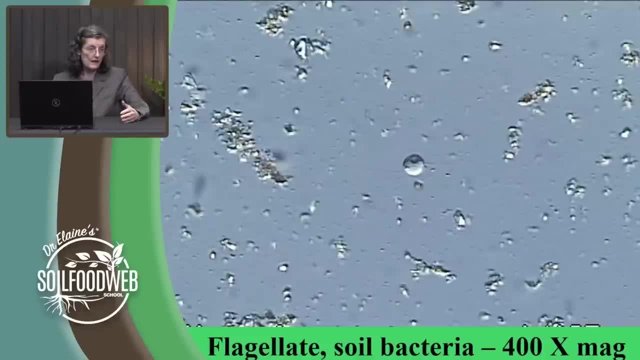 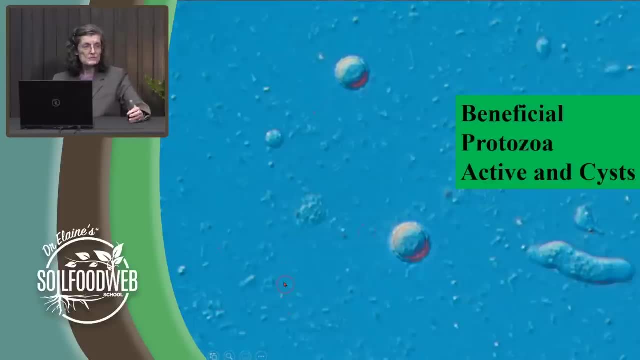 you start to look at everything that's going on in these pictures and those interpretations tell you that you something. so when you're looking at this picture, what would you say about the aggregate condition in this soil? not at all. they're about. the only aggregate you can find is this little. 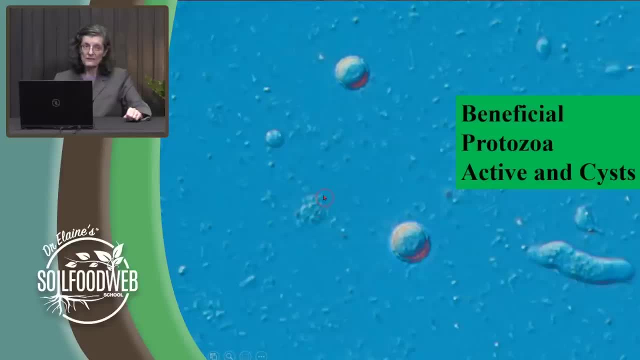 one right there and boy, this is. this is not good looking. now we have an active amoeba and it grows. you can see the clear tip right here. that pseudopod moves out first and then the rest of the body will come along. see all the little dots in there, don't they look exactly like the dots. 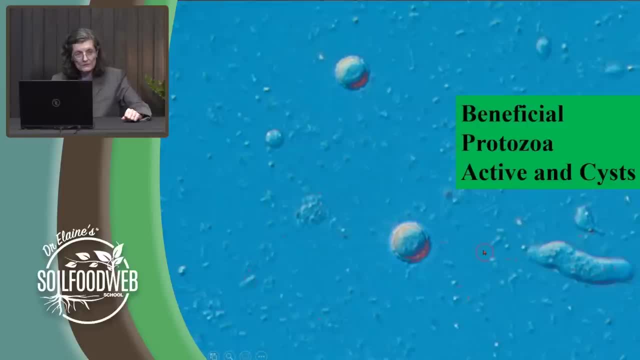 out here where all of these bacteria are hanging out. yeah, because these amoebae eat bacteria, and so there they are. they've got to eat 10,000 a day in order to stay alive and fat and happy, so she's happily chowing down, moving through the soil solution, eating every single bacterium that it likes. 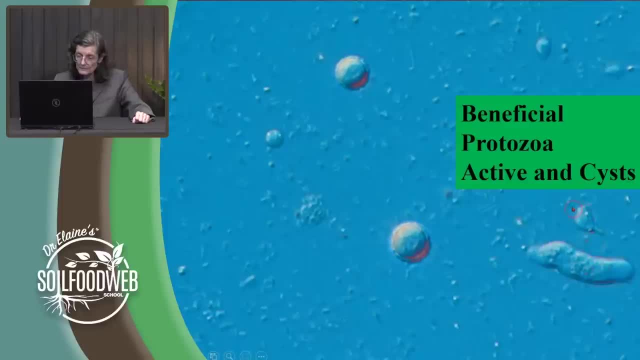 going through you can see another amoeba. it's a little, it's a different species. you can see this little tip that it's pushing out and that's very characteristic of that species of amoeba. you can see here cysts of the amoeba. they're always double walled and so the outer 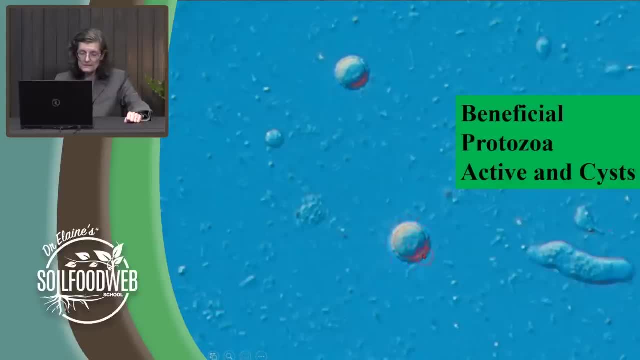 layer of that, that cyst is ornamented. When you look at this one same species, ornamented outside, not drastically ornamented, but definitely has a pattern, has a bit of a you know kind of scallop to the outside. Okay, now, how about this? Is that one of those guys? No, because it's not. 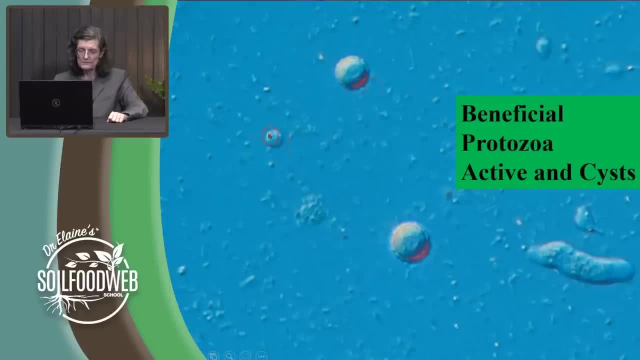 double-walled- it's only single-walled. Lots of stuff inside, Is it an amoeba? that's just kind of. you know, got a little tired, decided to take a little nap, so you stand and you watch this for 30 seconds and then suddenly you notice, oh, it's got a flagellum. This is a flagellate. 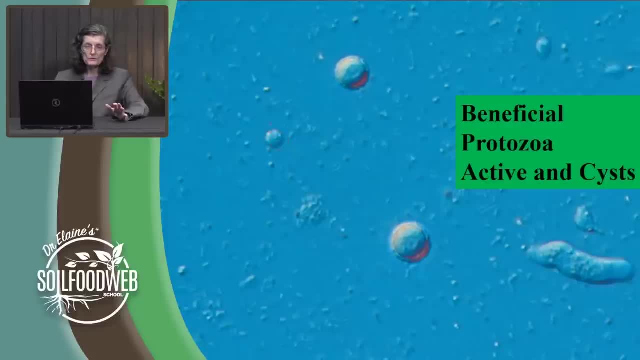 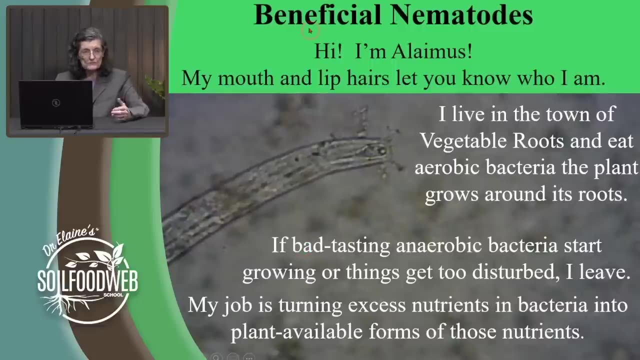 It just decided to take a nap for a while. Just because they're not moving doesn't mean they're dead, So sometimes you got to kind of poke them. So beneficial nematodes. we teach you the characteristics again of what the bacterial feeders look like. They all have. 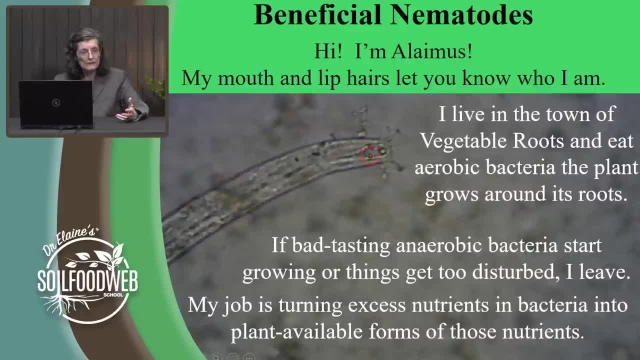 mouths like this, sometimes kind of wide V-shaped stomas, sometimes cylindrical stomas. We'll be looking for median bulbs and terminal bulbs and we teach you what the characteristics are for each group of nematode. So when we look at nutrient cycling- we've now talked about 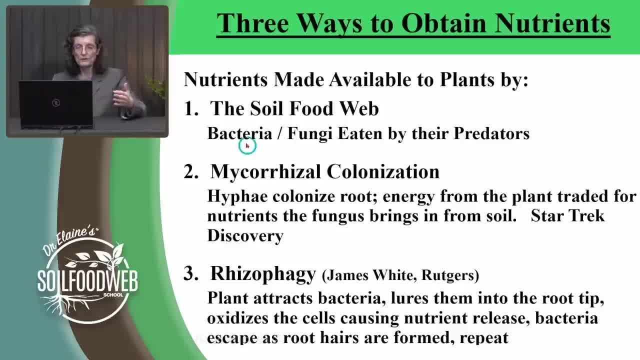 nutrient cycling in the soil food web, where the bacteria and fungi are eaten by their predators. We've talked about mycorrhizal colonization, where the mycorrhizal fungi are told to go get the nutrients that the plant requires and bring them back in exchange for more food. But there's 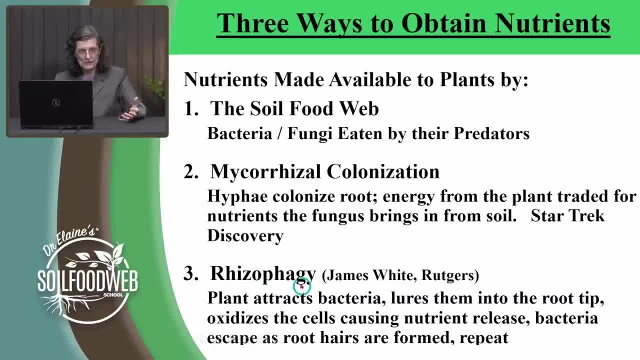 this new way that people have just started talking about, called rhizophagy, where the plant is attracting bacteria to the root tip And the plant lures those bacteria. they know what they're up to, They know what they're doing to the plant, They know how to. 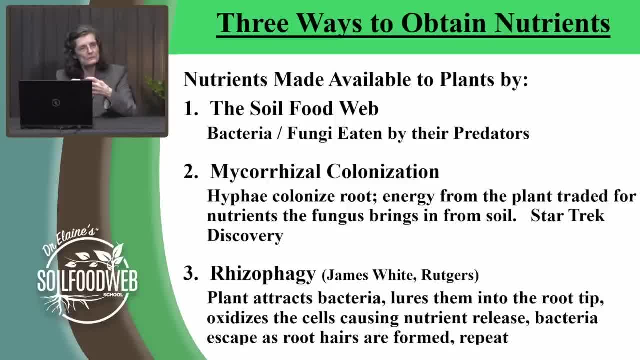 run a plant down So the plant just photosynthesize those bacteria inside that root tip. So the plant takes an oxidizing agent like bleach- the microbial version of bleach- And bleaches its root tips. so those bacteria can move into the plant root just right there at the tip And once all 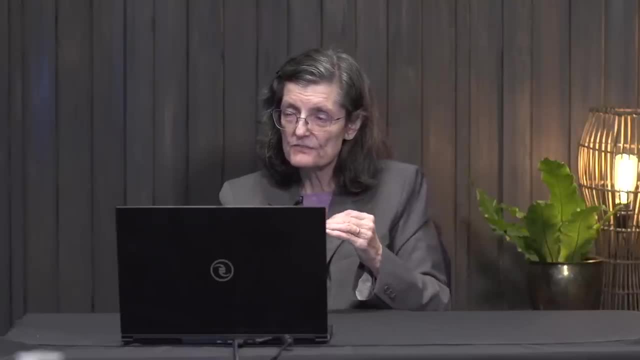 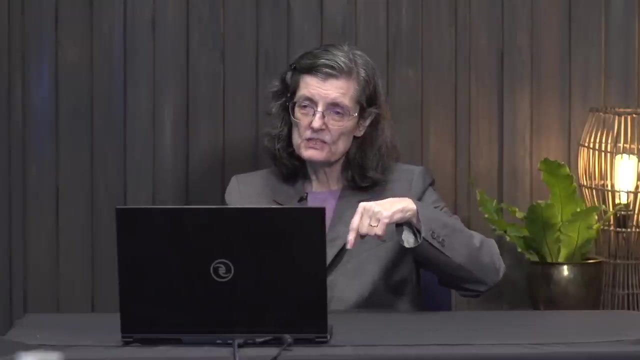 those bacteria have kind of gathered in that nice safe place, the plant sends out another wave of oxygen and bacteria. So you can see we have bacteria in all of this. Now you can see these bacteria oxidizing material and basically just completely decomposes the cell wall of those bacteria. which causes the bacteria to leak cytoplasm out of their bodies and into the plant sap. Kind of a clever way of doing that, getting extra nutrients by inviting these sweet, innocent, unsuspecting bacteria to come into the root system and then grabbing a lot of the nutrients away from. those bacteria. Well, so the end of the root tip of the plant is now closed off. Those bacteria follow the outer edges of the plant until they get to the root hairs that have started to develop, And apparently there's an escape exit right there where the root hairs start. So all those bacteria. 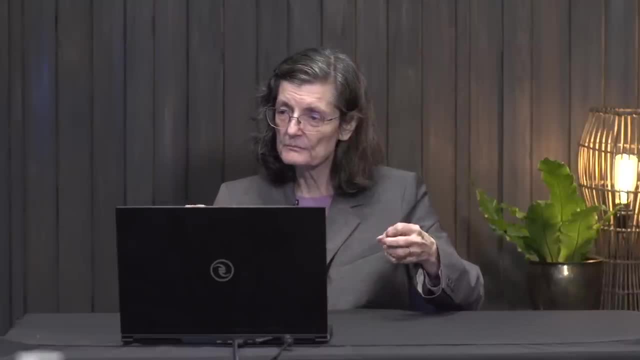 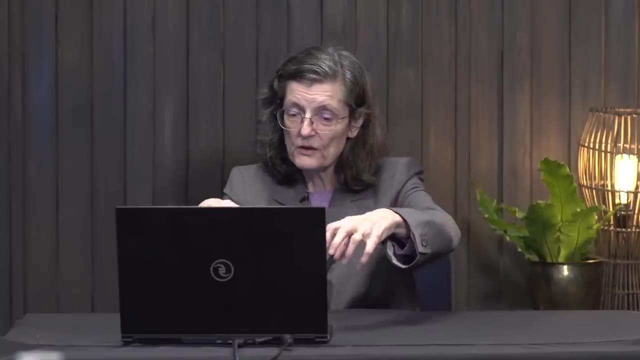 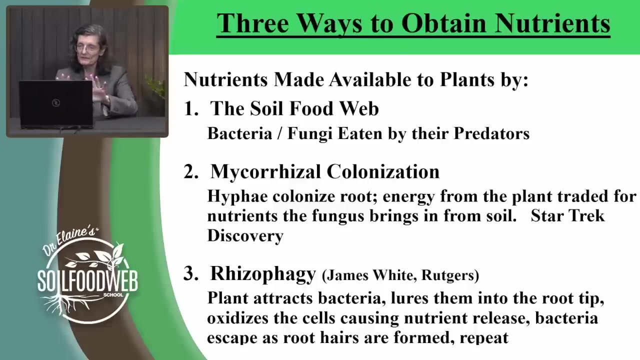 file out and they then start growing, taking up nutrients that are in the soil, regrowing their cell wall, and they go around back through the roots and hang out and wait until the rollercoaster opens up again And in the bacteria go. the plant then strips them of their membranes. 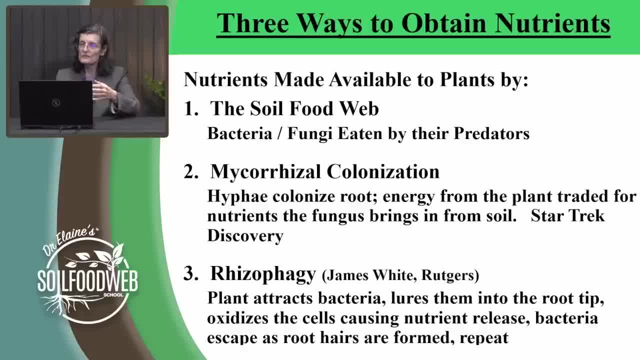 lose a lot of their nutrients into the plant sap and then the bacteria move back into the root system And then they go back around and go. It's kind of like me with a rollercoaster: Again, again, I want to go again, And they just seem to do that. And interesting only been brought. 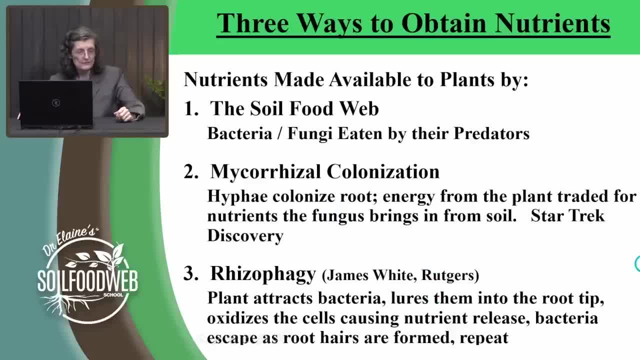 to light in the last, I suppose, you know, four or five years. So really interesting. There's yet another way for microorganisms to benefit that plant, And isn't it important to know that? So now, instead of just being the one mycorrhizal colony?